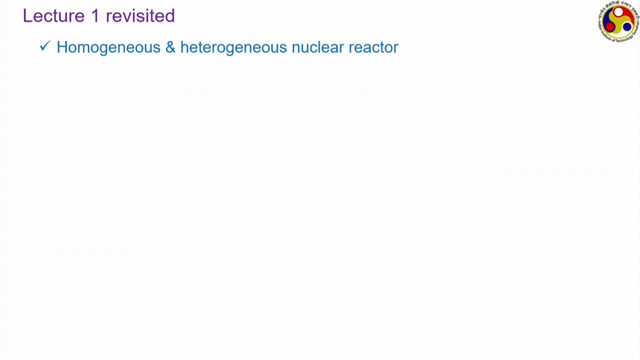 in the reactor we are going to get the same kind of chemical composition how? while homogeneous nuclear reactor has several advantages, but there are quite a few disadvantages also, particularly from kinetics and control point of view, And that is why the use of homogeneous reactors 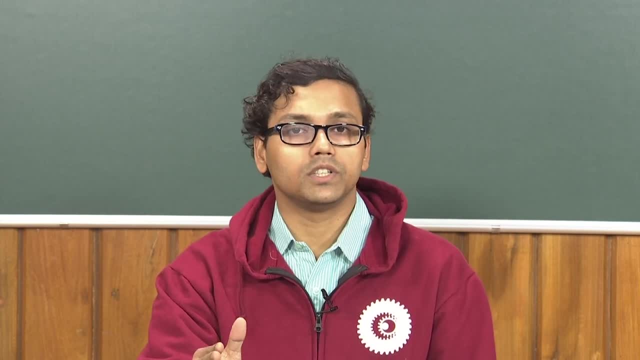 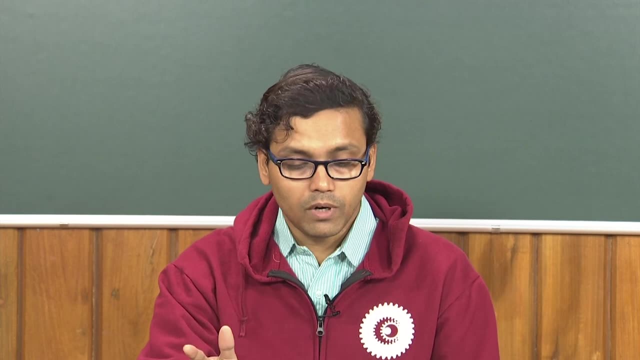 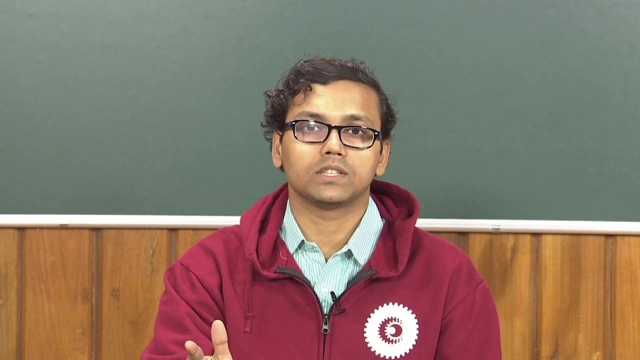 particularly the aqueous homogeneous reactors, Restricted to small scale applications such as a medical isotope separation or hydrogen production by radiolysis And for power generation purpose. we almost universally use heterogeneous reactors where fuels and moderators are placed as discrete elements, generally following: 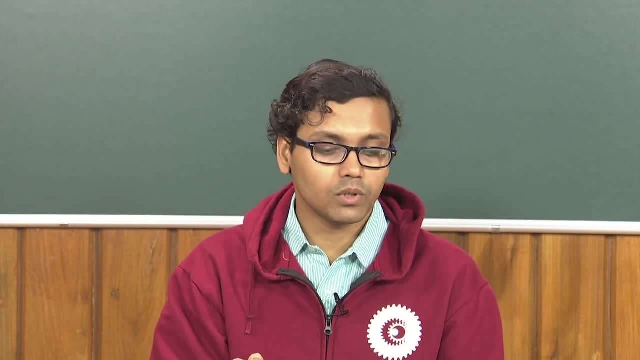 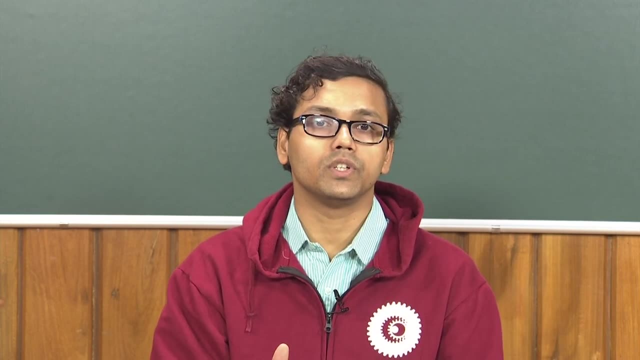 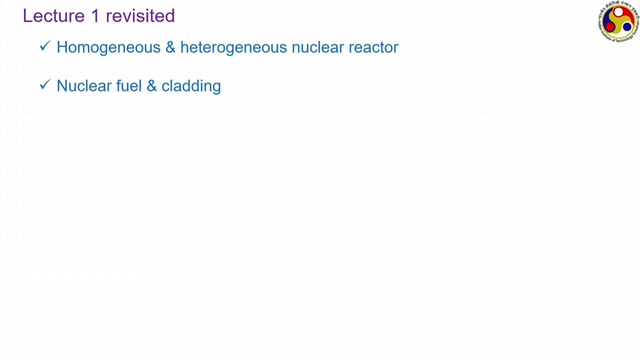 some kind of regularized pattern. We have also discussed about different properties of fuel and cladding, and now we know what are the desirable properties that we need to have for a fuel like high thermal conductivity, corrosion resistance characteristics, heat resistance, good mechanical strength at elevated temperature. Cladding has a big role to play. 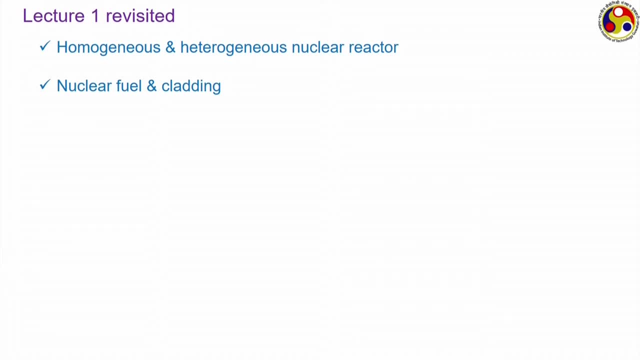 in the last point, that is, cladding is some kind of jacket which covers the fuel, thereby providing its structural solidity, And the cladding material should also have very low absorption, cross section and high thermal conductivity. Sometimes it can also provide some additional or extended heat transfer surfaces, particularly when we are using some. 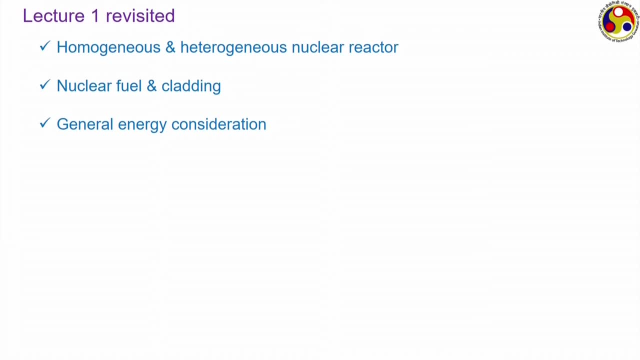 kind of gas as a coolant. Then we went to the general energy consideration and there we have seen that while generally more than 200 MeV of energy is produced for every fission reaction, we can get only about 75 to 80 percent of that transfer to the coolant. 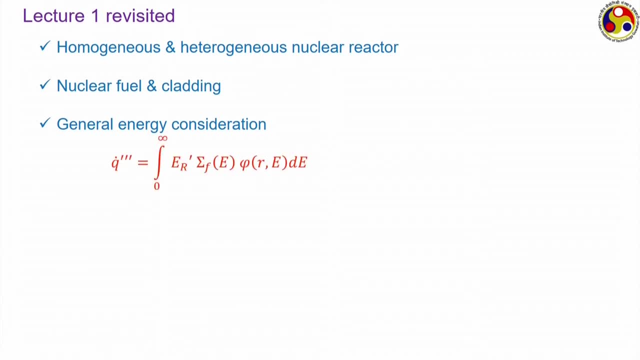 while remaining goes in the form of radiation. primarily The volumetric energy generation can be related by relation like this, where E? r prime is actually that effective energy that is available from a reaction and phi represents the neutron distribution. So this is the energy generation that we have seen. So this is the energy generation. 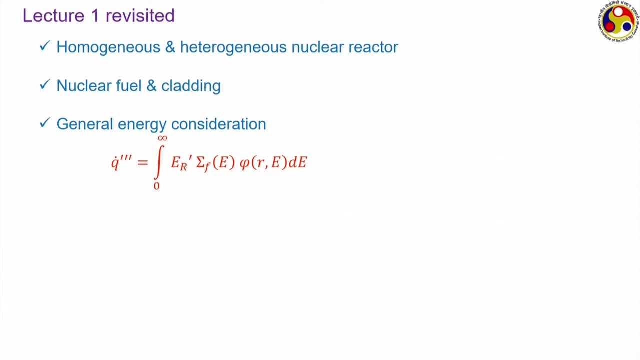 distribution inside the reactor. This is, of course, at a particular location, this integration is done. So in a way, you can also say there is volumetric generation that we are writing. this is actually a function of r. And then we discussed a specific case for a cylindrical 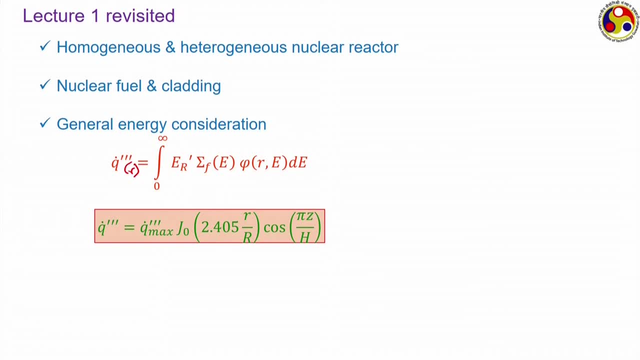 reactor which contains a large number of fuel, cylindrical fuel rods. Capital R is the radius of that reactor and capital H is the height of that cylinder. So this is actually the cylinder and accordingly we got this particular solution for this heat generation and it is. 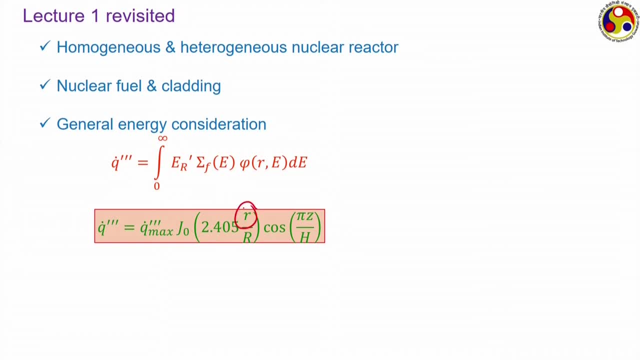 functions into a function of both r, which is a radial direction coordinate, and z, which is a axial direction coordinate. And finally, we have done the heat transfer analysis for two simplified geometries. Commonly in nuclear reactors, fuels are present either in the form of rectangular plates, very thin rectangular plates, and also cylindrical fuel rods. These 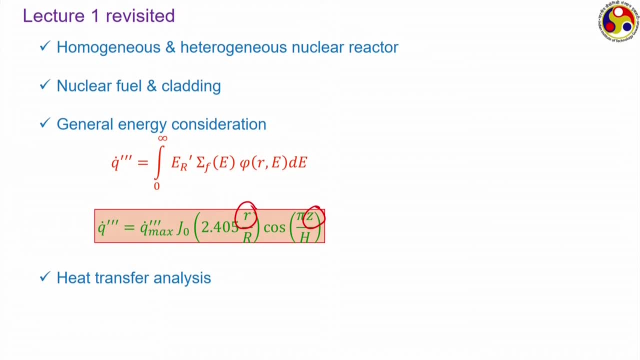 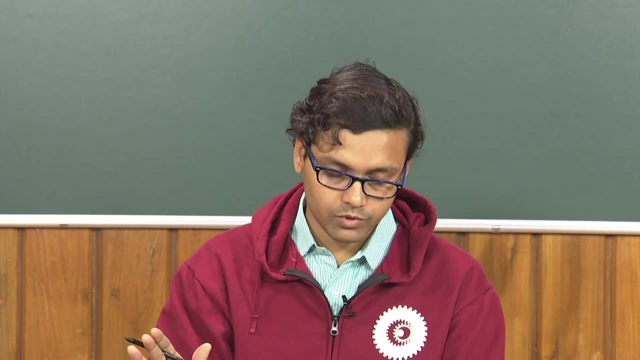 rods generally are such small diameter they are often referred as fuel plates, So they are not referred as fuel paints. So we have donequite simplified heat transfer analysis for both the cases by assuming constant fuel profit. sorry, constant properties for both fuel and cladding. 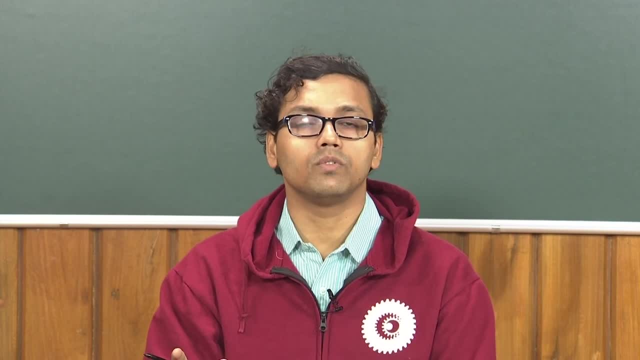 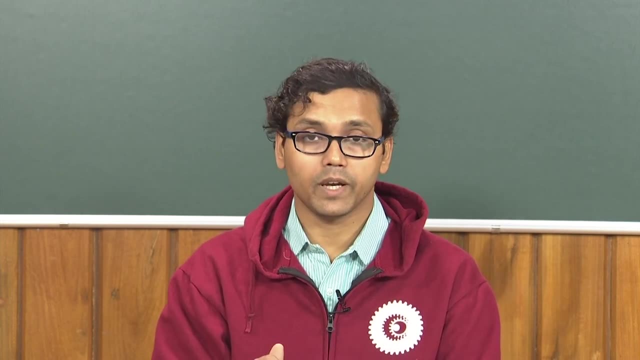 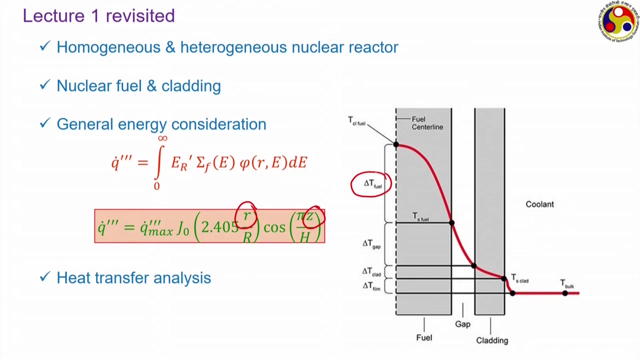 And also a very important assumption: by assuming uniform rate of heat generation throughout the reactor- And this was the solution that we have obtained for a plate type reactor- werewe can we have calculated this temperature difference that we may have across the fuel, and also the temperature difference we have calculated in 90 degree intervals From this. 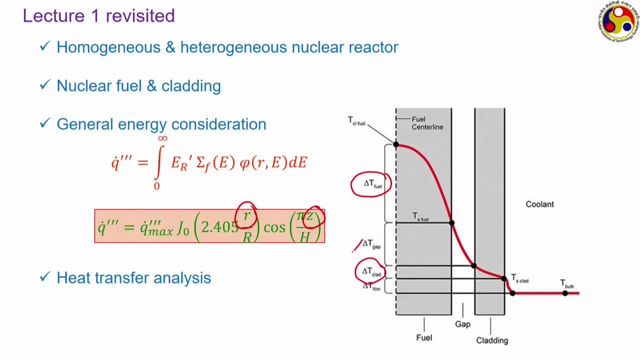 without any shapes and adaptation. we are getting, we are Ve4 raft and 5 rates Also we find may have across the cladding. This gap situation we have not analyzed but practical reactors may have a gap, also an air gap between the fuel and the cladding And also we have derived 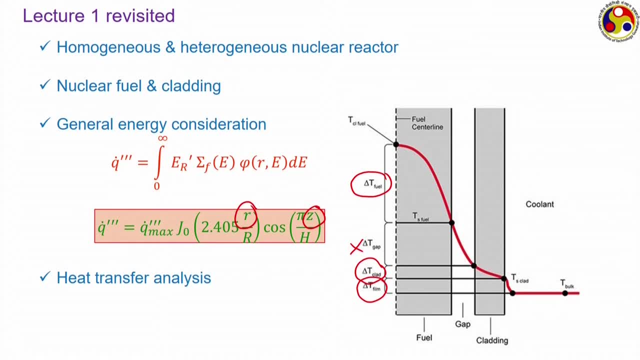 expression for this film: temperature difference, which is actually the temperature difference across the coolant boundary layer on the surface of the cladding. And we have also got by assuming some temperature value for the fuel centre line. we have got expression for the temperature at the fuel cladding interface, at the cladding outer surface. 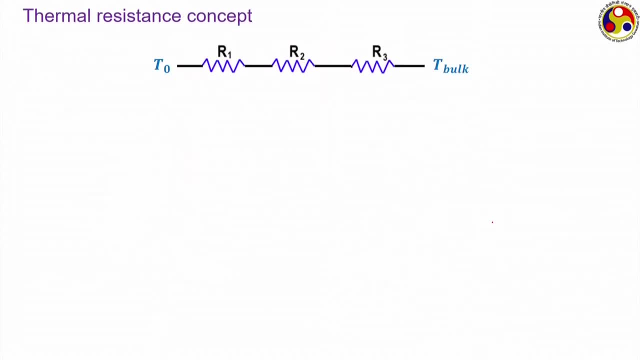 and also for the bulk of the fluid, And we have seen that primarily if we neglect the gap between the fuel and cladding, we can draw a simple electrical energy for that situation. where T naught is the fuel centre line temperature which can be thought about as a source of 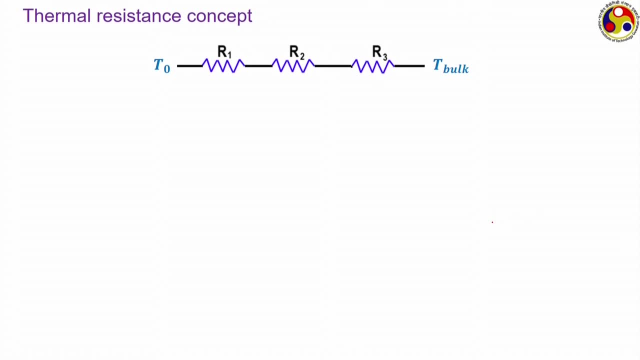 energy and T bulk is the bulk fluid temperature And in between there are three resistances through which the heat flux or rate of heat transfer- whatever we would like to consider- that is flowing through Here. q dot is the rate of heat transfer and R 1,, R 2 and R 3 are the 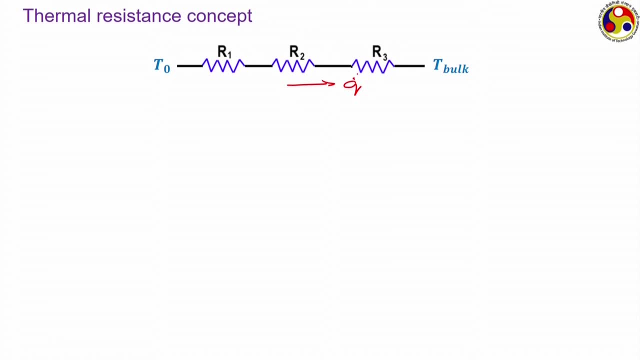 three resistances. R 1 is the fuel thermal resistance. R 2 corresponds to the cladding thermal resistance. Both R 1 and R 2 are actually conductive resistance because fuel and cladding generally being solid in nature, Liquid fuel can of course be there, as we have discussed. 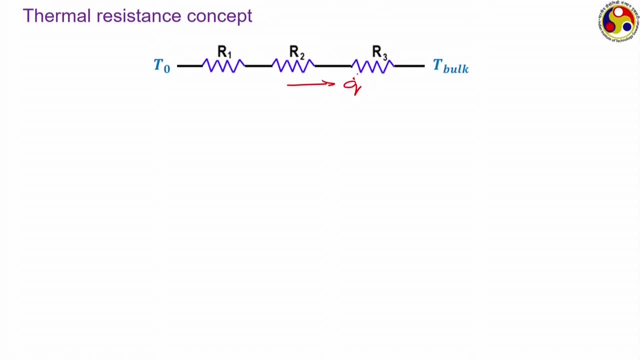 in the last lecture. but liquid fuel is primarily used in homogeneous reactors, whereas heterogeneous reactors primarily use solid fuels only. So both fuel and cladding are solid materials and hence R 1 and R 2 both refer to conduction resistances only. R 3 rather refers to the 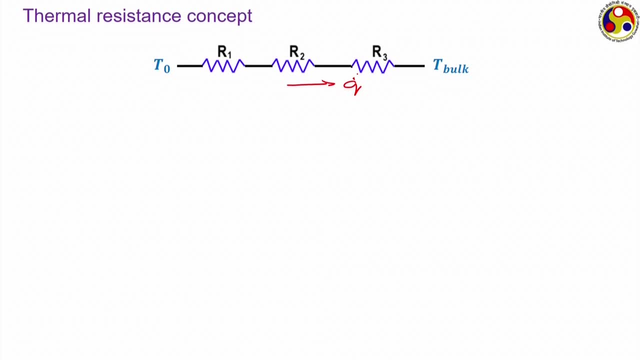 convective resistance because of the convective heat transfer that is going from the going between the coolant outer surface and the bulk of the fluid. These are the two geometries that we have considered: the plate type fuel and the cylindrical fuel rod. and these are the expressions that we got for the fuel resistance We just derive. 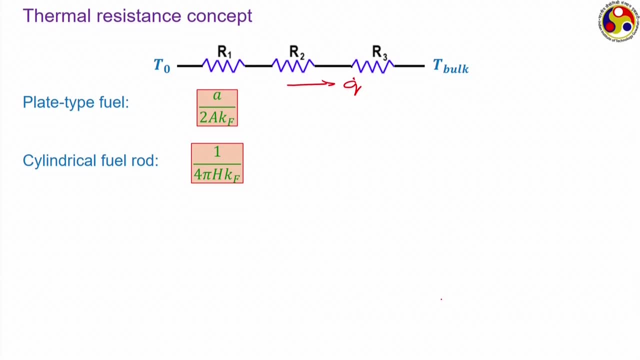 these expressions without doing anything else. So we have just derived these expressions without discussing into the details. We can clearly see that the resistance for both the cases at inversely proportional to the thermal conductivity of the fuel, which is a very logical, ah very, which is very logical re observation: Higher the thermal conductivity. 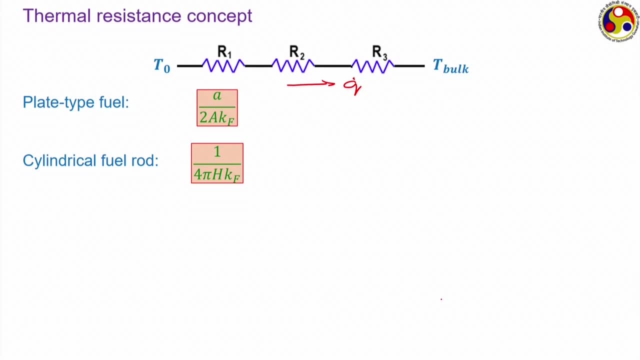 hence the smaller will be the value of this resistance and therefore the smaller will be the temperature difference across the fuel or the temperature difference between T dot and T s, which is the surface temperature at the fuel cladding level. So the temperature at the fuel cladding interface, the difference between T 0 and T s, will progressively be smaller. 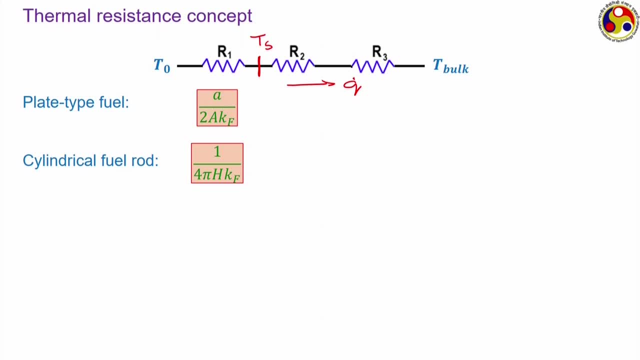 as the thermal conductivity of fuel keeps on increasing. That is why metallic fuels are highly preferable, So that we can keep the temperature differential small. but metallic fuel, pure metallic fuels or metallic alloys have their own disadvantages, like lower melting points, etcetera, If we use ah some oxide fuel or ceramic fuel. 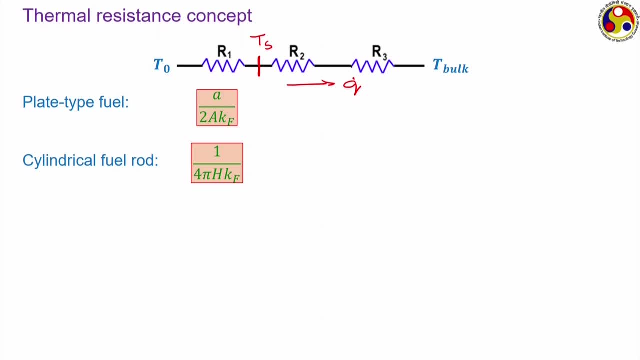 thermal conductivity will be quite low and we may have significant amount of temperature change across the fuel. Then the second group of resistance, which is associated with the conduction through the cladding. that is also inversely proportional to the thermal conductivity of the cladding. 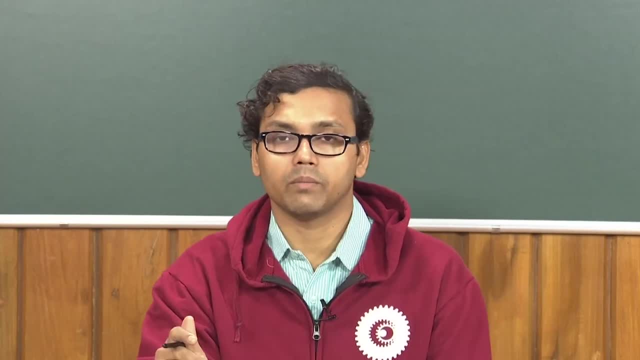 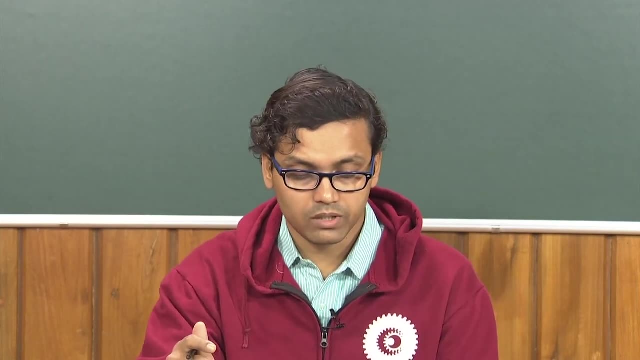 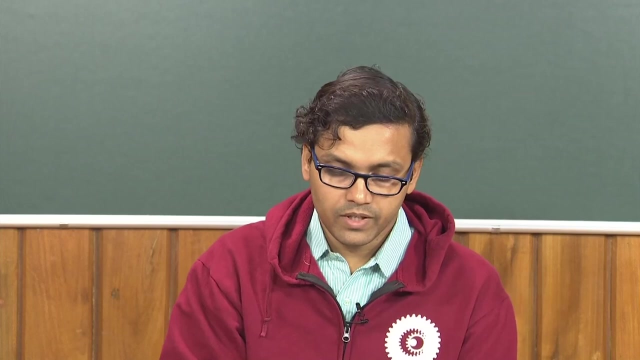 Now, cladding generally uses some kind of metallic element, like metallic alloys, like magnox or zircaloy or maybe stainless steel, which have quite reasonable values of the thermal conductivity, and hence the temperature change across the cladding itself is, ah, generally very small. 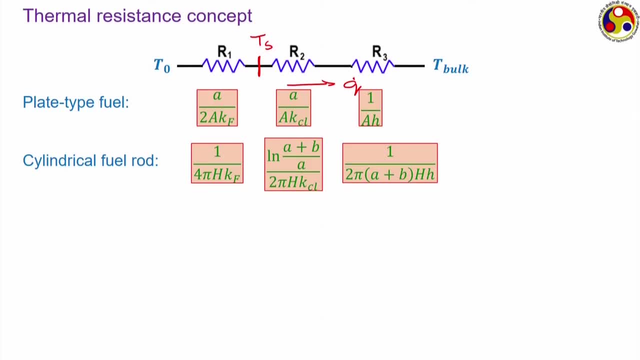 Then the third group of resistance, which is the conduction- sorry, the convection- resistance for the associated, the heat transfer from the cladding outer surface to the bulk of the fluid, and this, as expected, is inversely proportional to the convex responding convective heat transfer coefficient. 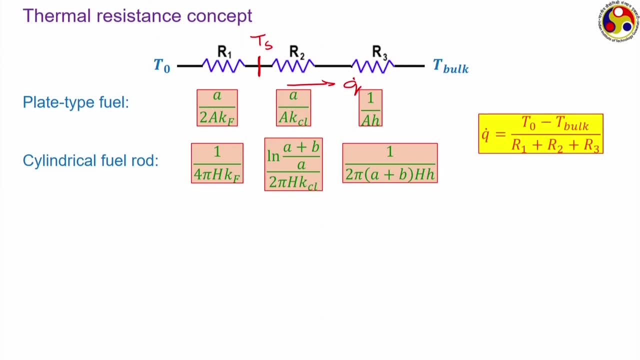 So for any of the elements, we can always write that the rate of heat transfer is equal to the effective temperature difference, which is T naught minus T bulk, divided by the corresponding resistance, ah, Ah And the, if we consider the case for ah, fuel rod. 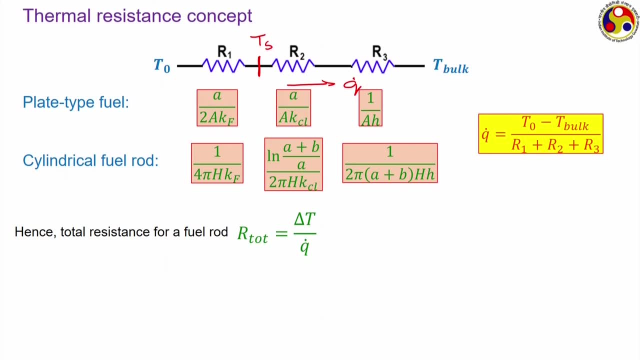 Ah, Yes, ç. then the total resistance has to be equal to delta T by Q. dot is the summation of these three components. The first one refers to the conductive resistance to the fuel. second one is the same for the cladding and third is, of course, the convective resistance. convective- 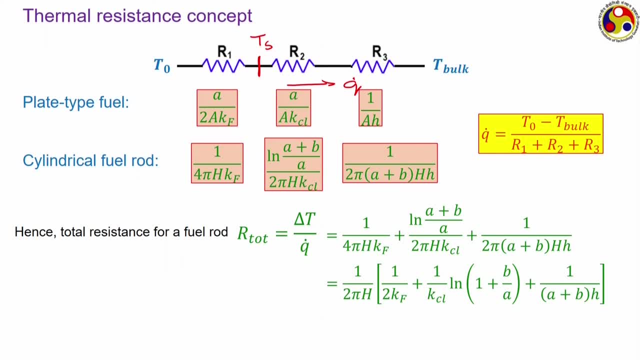 film resistance, we should say. So we can take 2 pi h outside the bracket and we get a simplified form. For most of the practical reactors, however, the thickness of the cladding is extremely small compared to the diameter of the fuel itself or radius of the fuel itself. 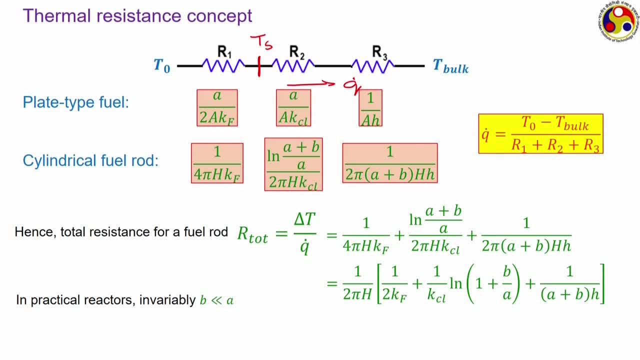 Fuel pins are also having quite small diameter, but size of the cladding can be even significantly smaller than that. So whenever we are dealing with the situation where B is extremely small compared to A, we can perform a simple analysis. We know that log of 1 plus x can be expanded, as if x is sufficiently small, we can always write. 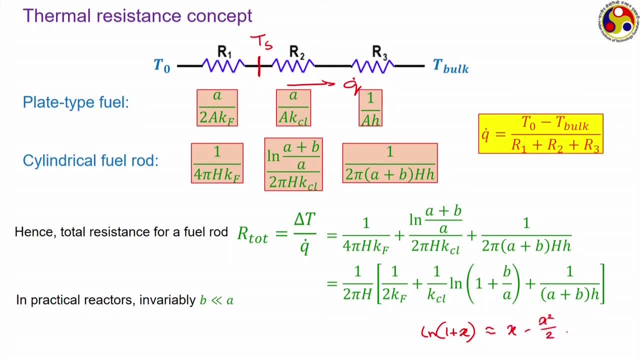 this as x minus 1.. Minus x square by 2 plus x cube by 3 minus dots. So in this case also, when B becomes smaller than A, we can write log 1 plus B y upon A to be nearly equal to B upon A Here. 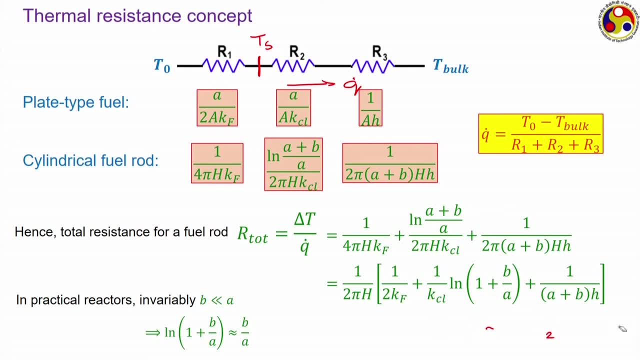 we are neglecting all the terms from second order onwards and accordingly, this equation simplifies to a simpler form like this: Now, this total resistance is quite important knowledge to have, Because this is the total resistance of the cladding. So this is the total resistance of the cladding. So this is the total resistance of the cladding. 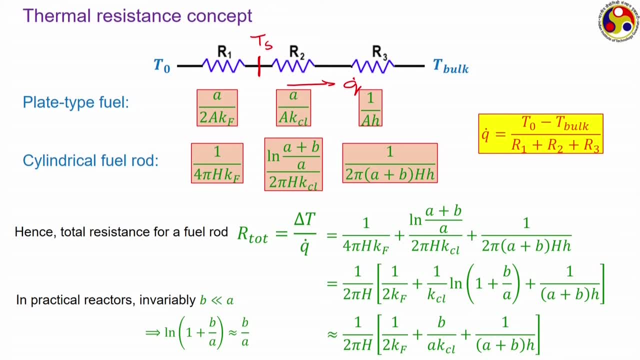 Now, of course, we have done this analysis using a very simplified form of the heat generation. We have assumed a uniform heat generation throughout the entire fuel pin or fuel plate element. However, that is not true in practice. There is always variation in the heat flux. 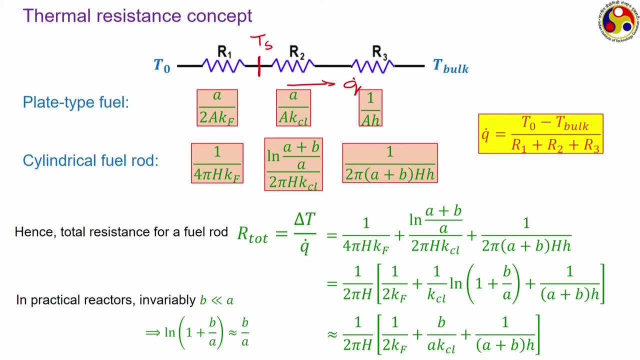 in both radial and axial direction for a fuel rod, But generally the dimension in the radial direction is so small compared to that in the axial direction we can invariably take the temperature variation in the radial direction to be negligible and consider only the axial directional variation, And in that case this concepts of thermal resistance is. 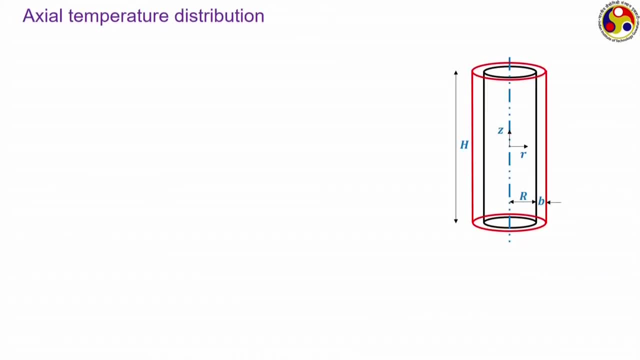 very important. We shall be seeing that in this particular case Here our geometry is that of a cylindrical reactor. Here, actually, the diagram is not perfectly placed. I can say: This is a fuel pin that I have shown here. A fuel pin is: 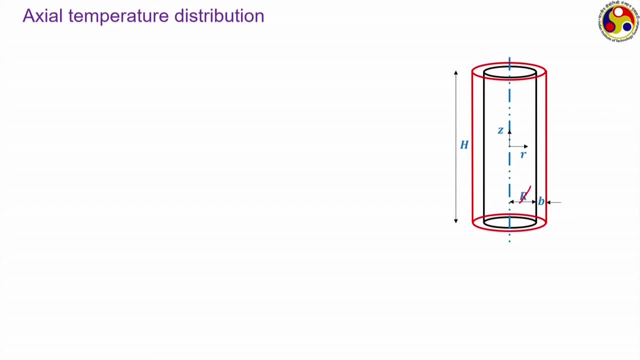 a fuel pin which is having this r is wrong, which is having a radius of a and the corresponding thickness of the cladding is b. And here now, instead of 1, we are taking 2 dimensions: r is the radial direction and z is the axial direction. 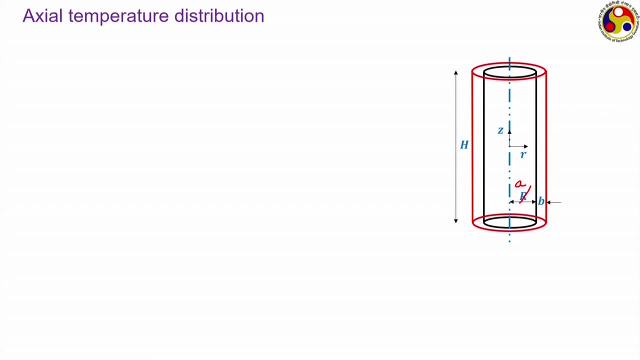 And our centre, or the origin of the coordinate system, is located at the centroid of this particular fuel pin, That is, we can say that the expanse of the fuel pin in the radial direction, So this from r equal to 0 to r equal to a, whereas that in the axial direction is: 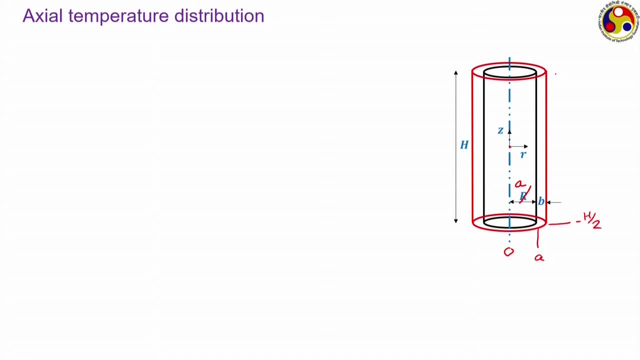 from some minus h by 2 to plus h by 2, as h is the total height And this particular location. sorry, let me correct this. this particular location refers to z equal to 0, And now this is the fuel pin that we have, and we are placing this fuel pin inside a large cylindrical. 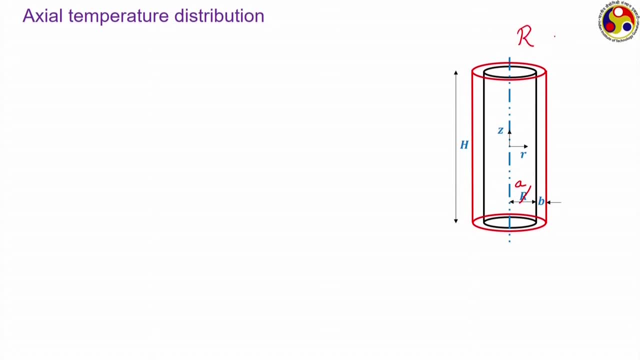 reactor of radius, capital R and height as the same height of the ah of each fuel element, which is capital H. Now we have earlier analyzed such a situation and seen that the in the last lecture we have seen that corresponding distribution of the volumetric heat flux can have a form like this. Now, if we apply this equation to a, 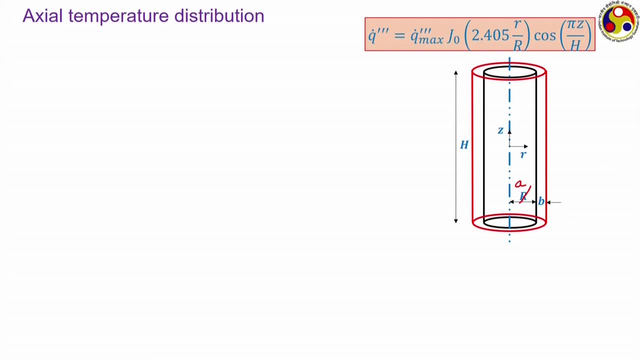 fuel rod which is located just at the centre of the coordinate system, just like this one here. That means it is located a position at r equal to 0 and so ah, invariably, we can reduce this one to a form like this: That means the heat flux becomes a sole function. 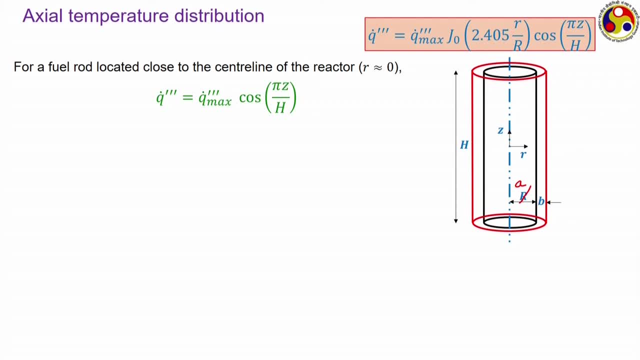 of z but ah. this is applicable only for the fuel rods which are located quite close to the origin, that is, at r equal to 0.. If we are talking about a location which is ah, which is not very close to the centre line, then q, then in that case we can also write. 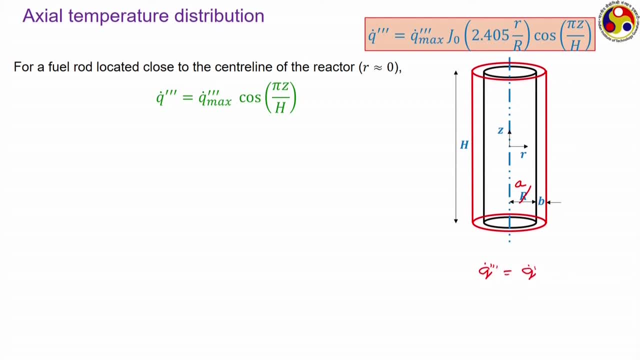 ah. q dot triple prime is equal to q dot triple prime max, which is a function of r. into this cos pi z by h, where this q dot max will keep on varying in the radial direction and for different radial location we are going to get different value for this maxima. But presently 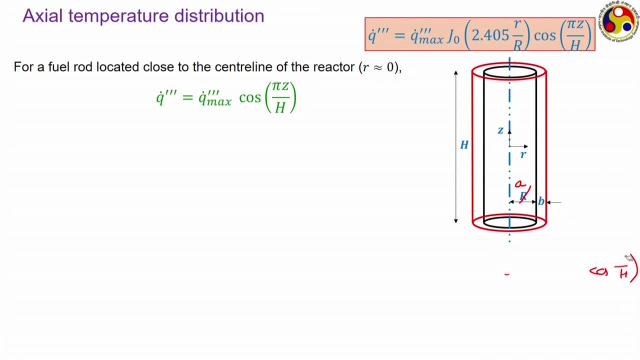 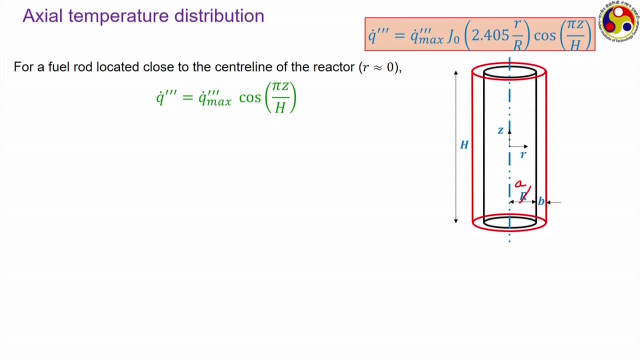 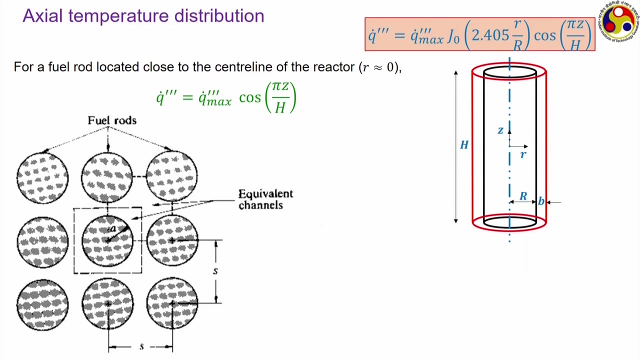 be neglected And hence for that particular fuel element, this ah heat generation becomes a sole function of the axial directional coordinate which spans from minus h by 2 to plus h by 2.. Now in a practical reactor, quite often you will find that the fuels are having an arrangement. 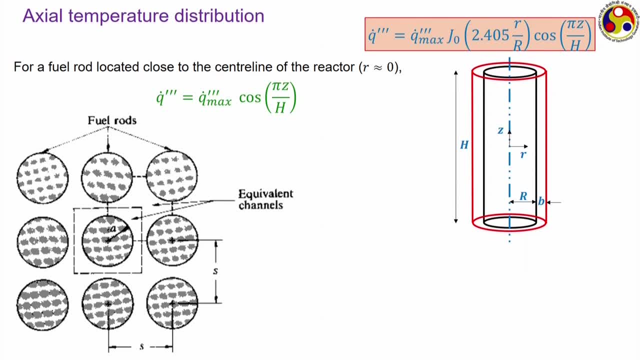 like this. They are generate paste in a lattice like this, where the these are ah. this circles are all fuel rods, Like 9 circles are shown here. each of them is ah. each of them is a fuel rod. So there is a mixture of e to m which, in principle, it is being therefore attacked. 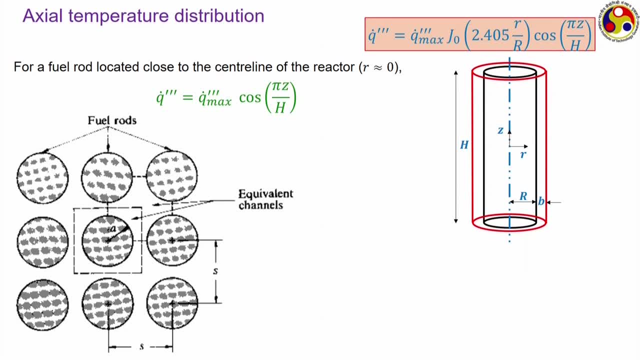 plus h by 2.. Error is fossilized again. after this. there is no partial加 on a rotation fuel rod, and all of them are immersed into thelarge expansion of coolant. So so there is no exclusive coolant channel. the coolant is only flowing through the intermediate spaces. 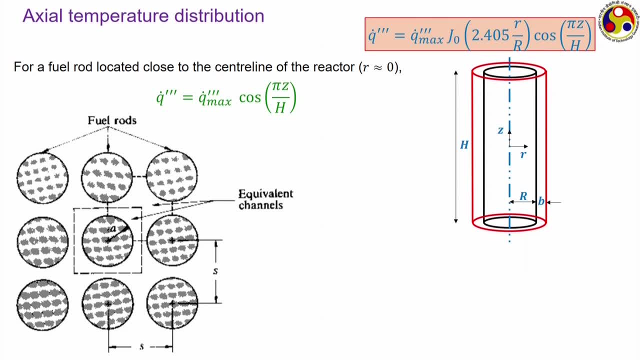 between this fuel pin. Now we, instead of considering all this coolant channel or all this fuel and coolant flow around that, let us just consider one and use the corresponding symmetric condition with respect to the other. So here each fuel rod is having an radius. 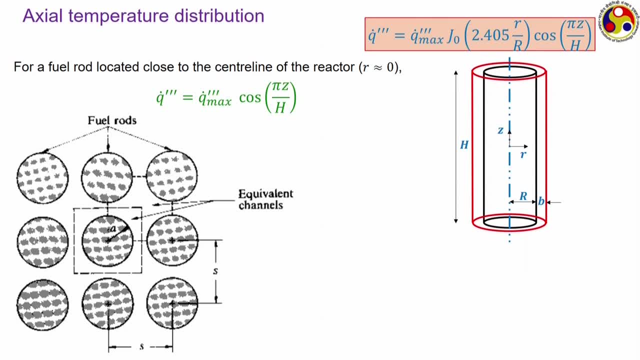 of A and around each of them we have considered a square of size S. Here S is the spacing between twoneighboring coolant fuel rod, in both directions, So and S is also the size or dimension of this particular square block that we have selected. 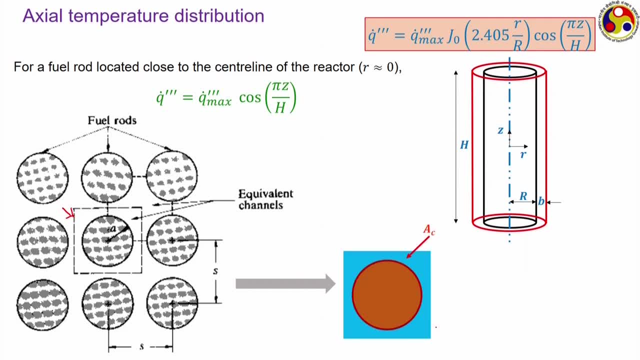 So we can be visualized to have a formula Form like this, wherewe have our domain reduces to a square block which is being filled up with water and theta or whatever coolant we are may be using, and also there, at the say, around the central end of that, we are having a circular fuel pin which is having a radius. 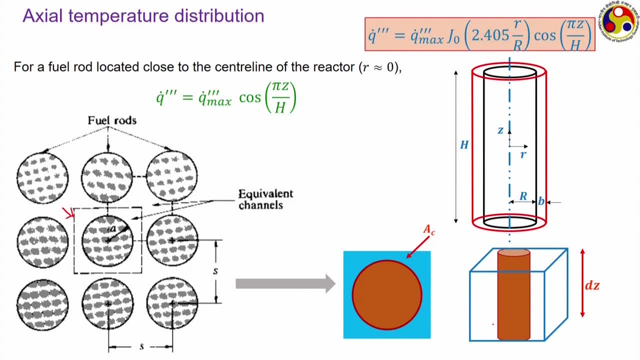 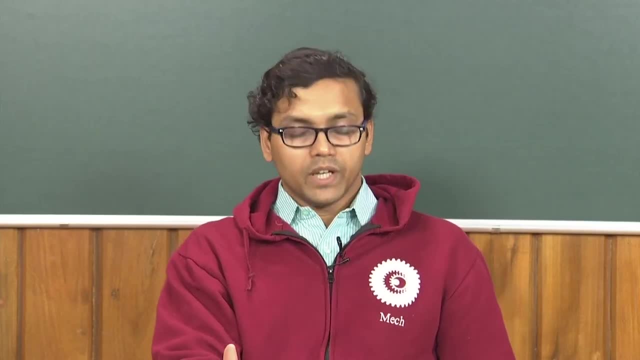 of A. This is the view from the other direction. Here let us consider an infinitesimally small portion of this particular fuel rod, Fuel rod and surrounding coolant, which is having an height of dz. So if we apply an energy balance, whatever amount of energy that has been produced by this particular fuel, 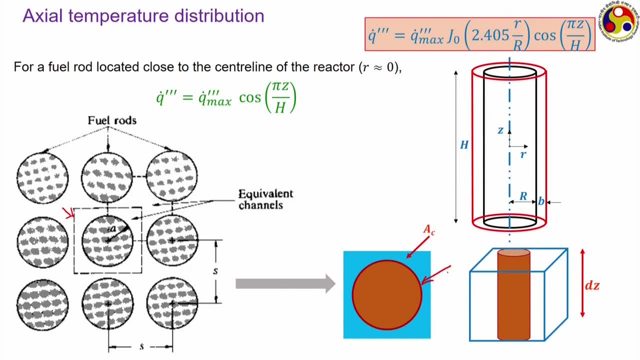 element, over which is having, let us say, the fuel element is having cross section area of f and its height is dz. So over this volume of A, f into dz, whatever amount of energy the fuel releases, the entire amount of energy can be visualized to be consumed. 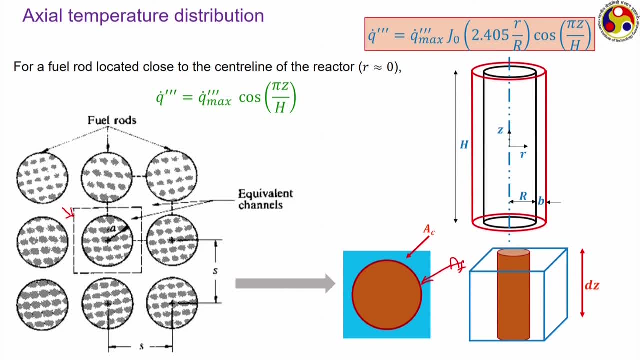 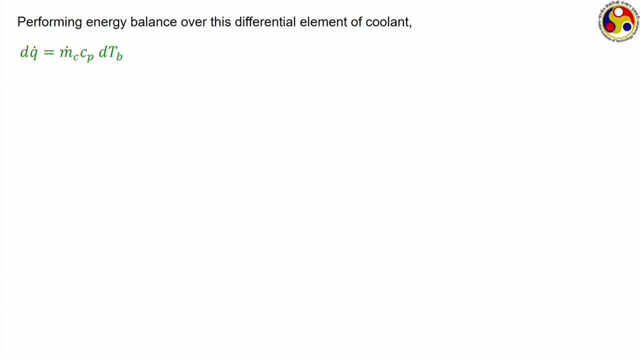 By the fluid which is restricted in this area A, c. accordingly, we may write this particular energy balance equation, where d- q, dot is the amount of energy released by the fuel element over this small portion of dz, and this is the corresponding temperature rise of this fluid. m dot, c is the corresponding mass flow rate and d t- b is the temperature difference. 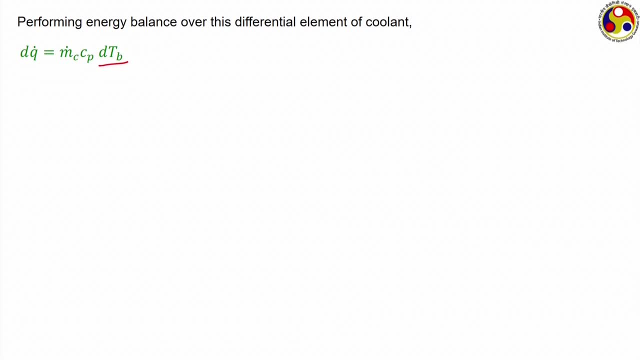 of the, the temperature difference, the fluid experiences while passing through this, passing through this infinitesimal small time of dz. Now, d, q, dot can be visualized as the. instead of writing power, we can consider this one to be the volumetric power multiplied by the total area of the heat transfer surface. 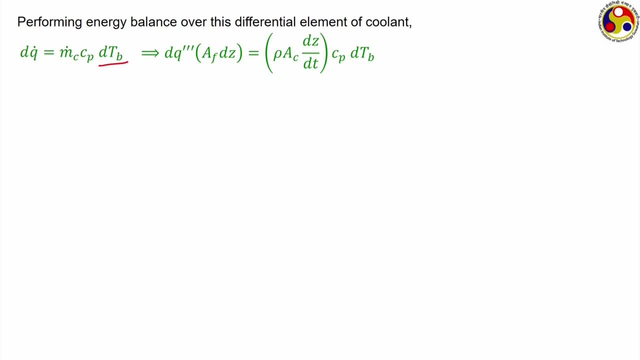 So here the heat transfer is taking place from the fuel towards the surrounding coolant, and in this case the effective area has to be the fuel surface area, which is A, f. And now, on the right hand side, we can expand this mass flow rate as the product of rho. 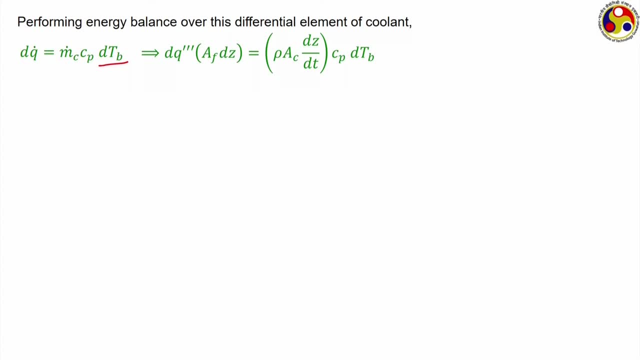 and the corresponding cross section area of the channel in and the velocity. but it is not necessary. also, if we rearrange that using the original form, then the temperature difference of the fluid across the channel comes out to be this particular form. and then, if we put now the expression for the heat flux, which is of course a- as we have neglected- any kind. 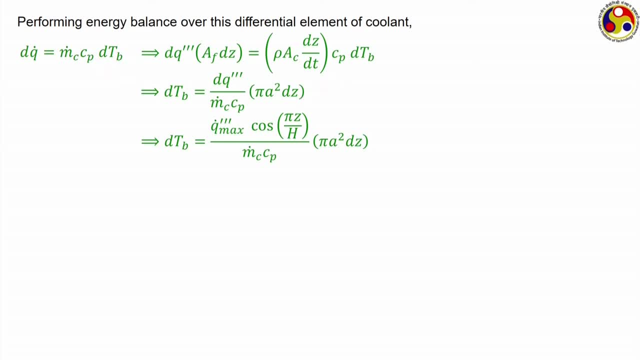 of radial variation. So the radial variation that remains is in the axial direction, which is following cosine function and therefore this temperature difference is also found to be a cosine function. We need to integrate ah this function from the inlet of the channel till the end of the. 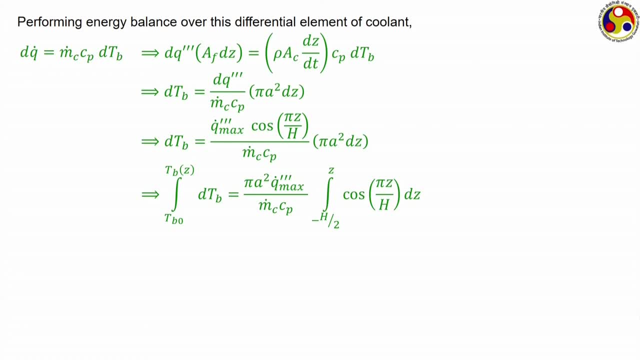 channel or maybe till some intermediate location, so that we can calculate the temperature of the coolant at that particular location. So this is where we are performing the integration: from ah, some minus h by 2, which refers to the inlet of the channel, to z, which can be: 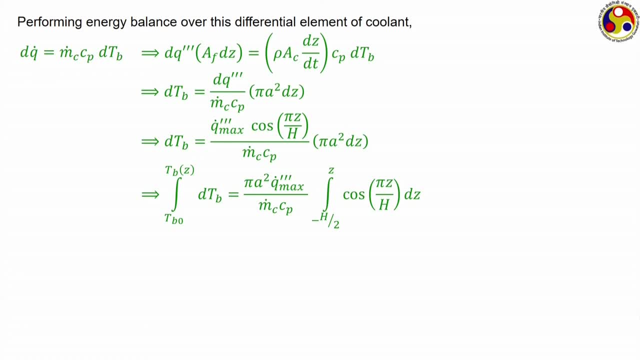 some arbitrary location inside the channel and corresponding temperatures are: d t b naught refers to the temperature at the location h naught, or I should say minus h by 2. d t b naught refers to the. this refers to a temperature of the coolant at this particular location. 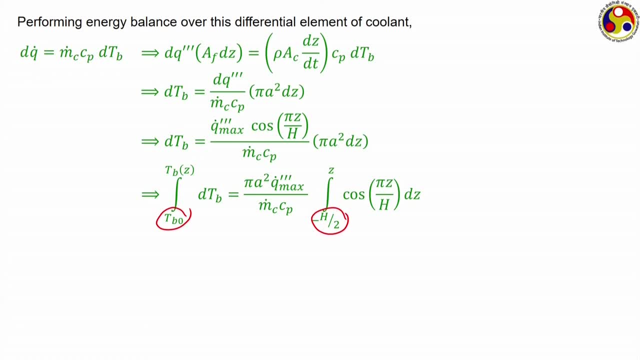 which can be visualized as the inlet to the channel. So, after performing this integration, this is the expression that we are going to get where, ah, we are having t b naught. So, ah, inlet temperature for the coolant, and then some constant terms and finally, 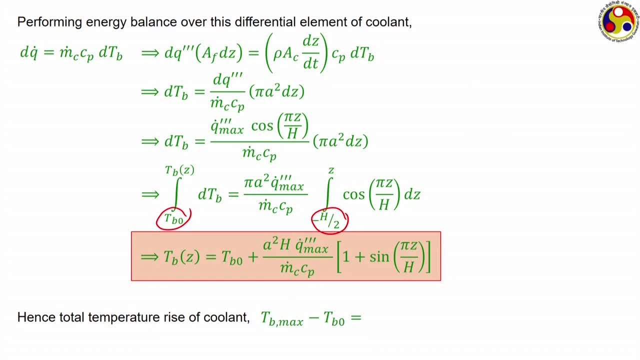 a sinusoidal component. Here, the total temperature rise of the coolant can be obtained by putting minus h by 2 in the above equation, and ah. hence that again. ah, bring some sort of this again. ah, it is some sort of constant, as you can see, if we do not consider the radial variation. 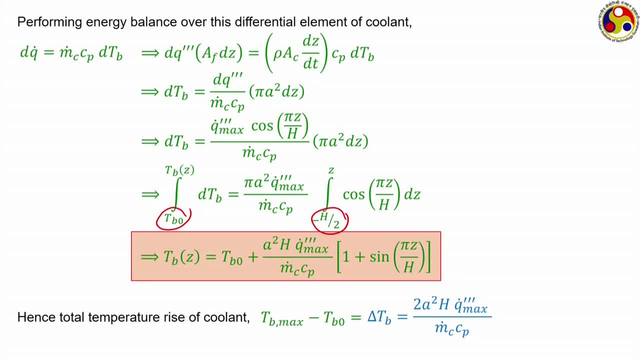 in the channel, So we are having the maximum heat flux. other terms: all are constant, and here this numerator can also be replaced with the term v rod, where v rod refers to the volume of each fuel rod. Now, how it can be a volume of each fuel rod, that should be the cross section area of the 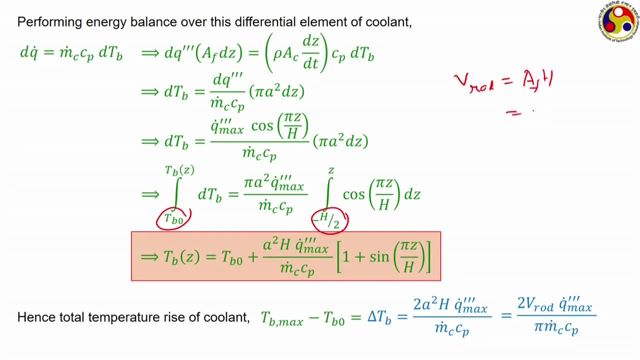 fuel rod into h and its cross section area is pi square into h, So the the term a square h. this equation can be replaced by the volume of the rod divided by pi, which exactly we have done here. This is the total change in the coolant temperature during its passage. 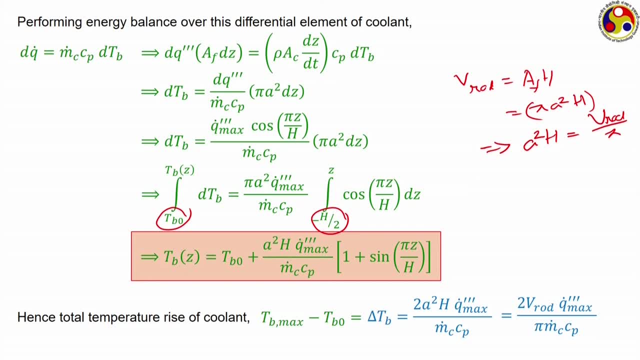 from the passage to the reactor, and if we use this expression for this total temperature rise, then the temperature profile for the coolant can also be written in a form like this, and also the term beta that we are using as an abbreviation. that is nothing but pi. 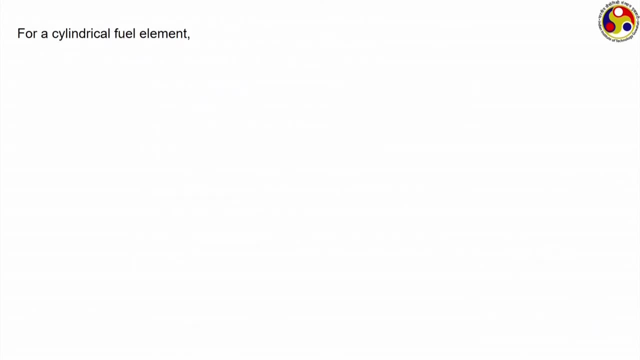 by h. So for a cylindrical fuel element, now we know that the temperature difference across the coolant film, that is, temperature at the cladding surface minus the bulk fluid temperature, is something like this. Now, if we use the concept of the, this is the concept of the. 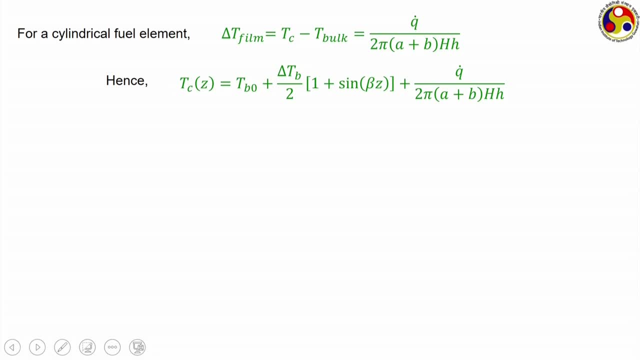 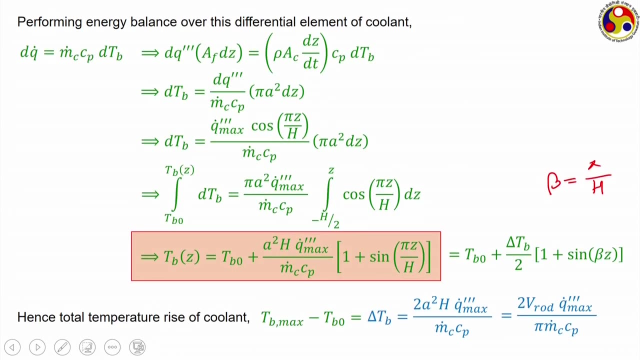 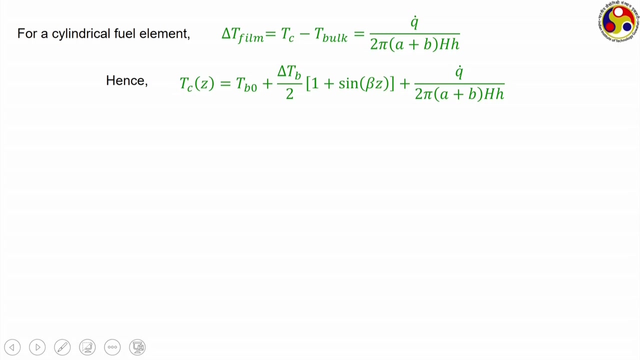 thermal resistance. So if we put the expression for T, c or a, rather T bulk, into this which we have just obtained- the previous slide here, this- then we can get this particular expression which here, which can be simplified by putting the expression for actually not simplified, we can expand this: the q dot, the rate of heat. 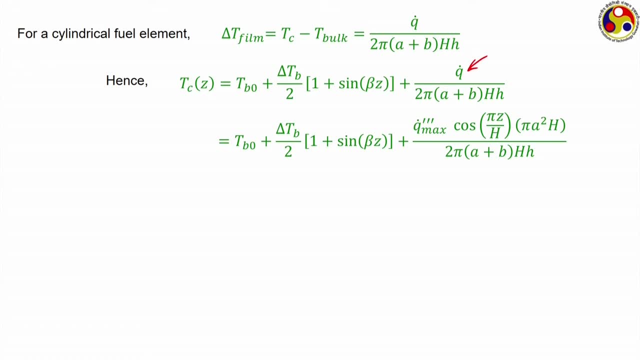 transfer that is there, that has been replaced by corresponding cosine term and finally we arrive at this, That is, the variation of coolant temperature in the axial direction can directly related to the coolant inlet temperature and the, the sine and cosine term, with beta in as one of the coefficients, or beta in the in the bracket. 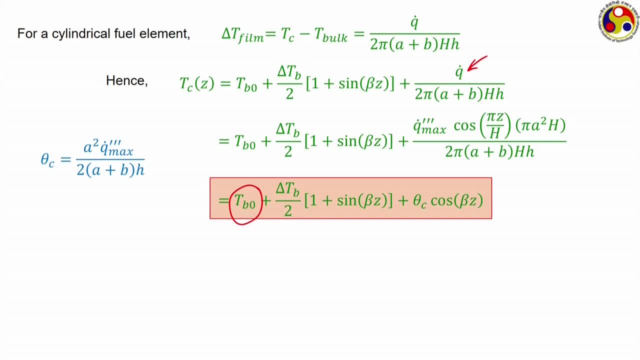 Here this theta c is actually a shorthand form that we are writing, which is equal to a square into q, triple prime, dot max divided by twice a plus b into h, In short, these sto Holder signature. here, this property we have achieved, which we have used only to give this equations, is slightly shorter. 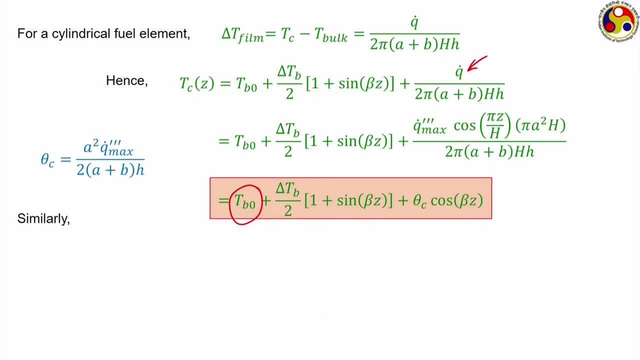 Similarly, we can also calculate the temperature at the interface between Fuell and cladding. that is exactly- there has been attempted to this- the centraline temperature. Similarly, we can also calculate the temperature at the interface between Fuell and cladding, and also you can calculate the Fuell. 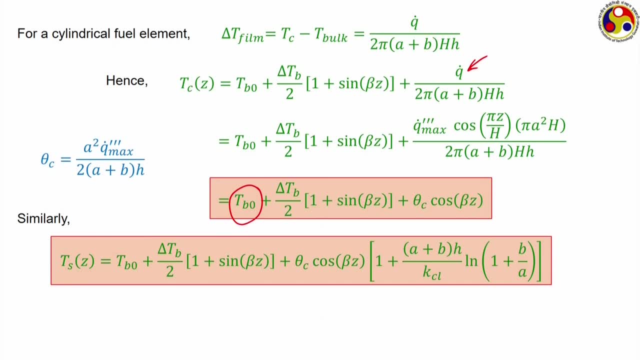 and also you can calculate the Fuell and cladding exactly have been attempted to you. so that is exactly where that hometown, in detail: wellpops Water, K Oil Processed in quero Pac. These terms locks, These terms sin. we have two different resistances coming in. this one corresponds to the film resistance. 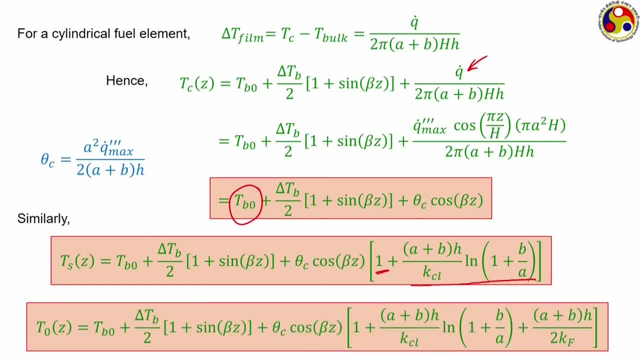 and this one corresponds to the cladding resistance. And finally, if we write the expression for T naught z, which is actually the temperature at the center line of the solid, then we get the same form, but now we have three electrical resistances. while this one corresponds to: 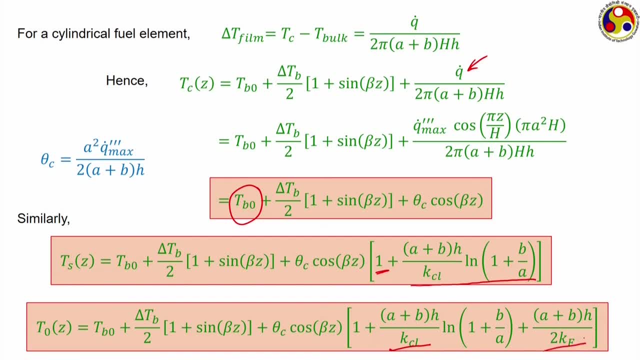 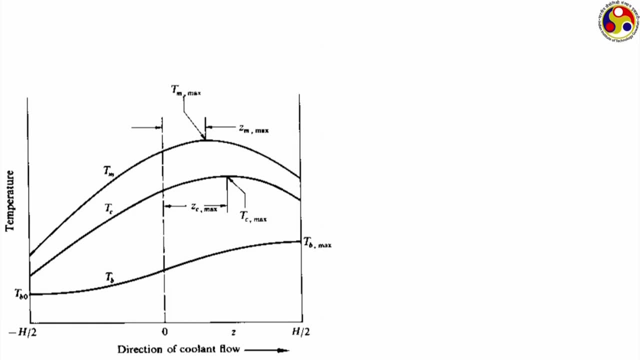 the cladding. this one corresponds to the conductive resistance for the fuel, And this is the typical temperature variation that we may find comport a cylindrical reactor generally, While this one is for the coolant. this is, this is the inlet of the channel. 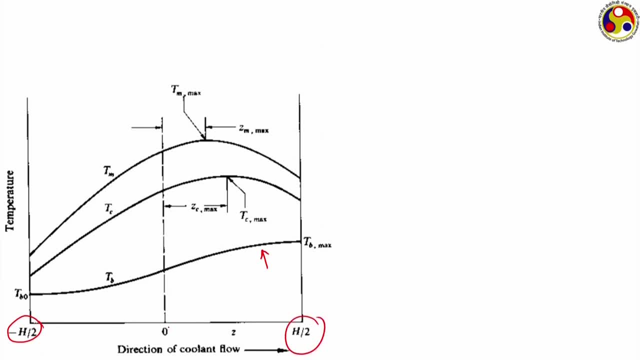 this is the exit of the channel and this is the center line in the axial direction. So as we move towards the exit, the coolant is getting more and more energy, increased amount of energy because of the fission energy release And hence the coolant temperature continues. 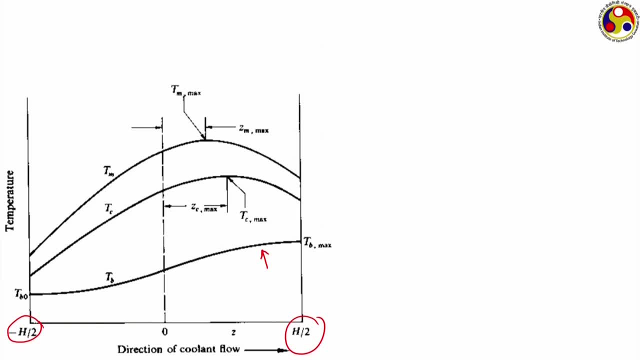 to increase, unless, of course, it reaches some temperature, some prescribed value. However, that is not true for the other two temperatures of interest. one is the center fuel center line temperature and other is the cladding surface temperature. This T m refers to actually fuel center line temperature, as per our terminology. You can: 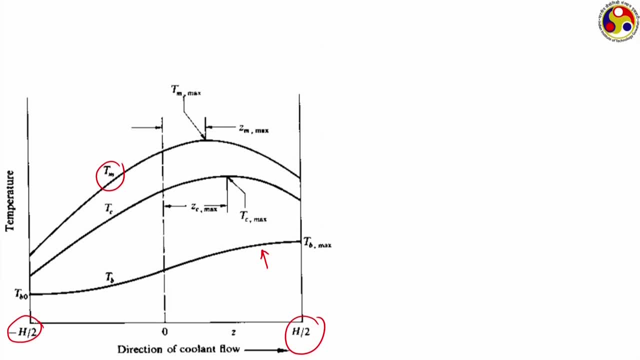 see both the cases. both or both the profiles show a maxima. So the location of this maxima for the cladding surface temperature can be found by setting that d dz of cladding temperature to be equal to 0, which reduces to a form like this, and after performing the differentiation: 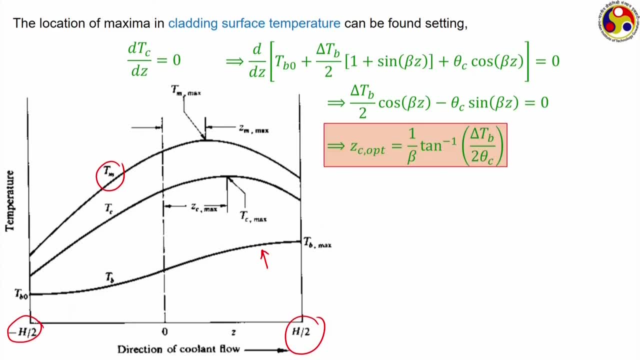 we are having this and finally we get the location of this optimum- look optimum- cladding surface temperature. Similarly, you can also calculate the location of the optimum fuels center line temperature, that is, by setting d, t, f, dz equal to 0 and corresponding form. 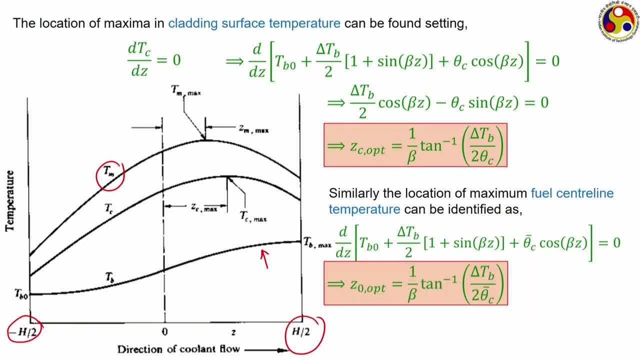 is this and we get z. So this is the center line. optimum value of just center line equal to 1 by beta into tan inverse delta T p by 2. theta bar C: Here theta bar actually is a shorthand notation because as there are quite a few terms involved, three different resistances involved during. 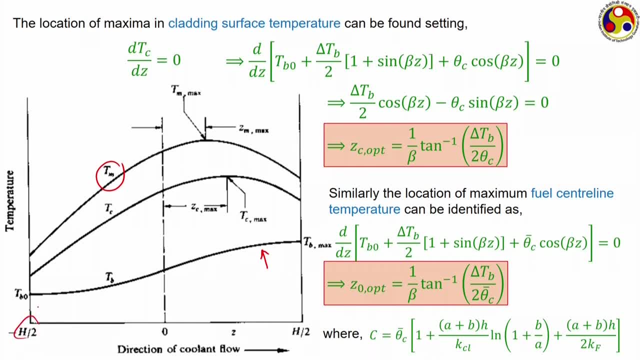 the calculation for the fuel. we consider them in a short notation of. actually there is a typing error here. Here, this is this: This is this theta C bar that I refer to, and this should be theta C that we are using from from the earlier slide onwards. So this way we can calculate the optima for both the 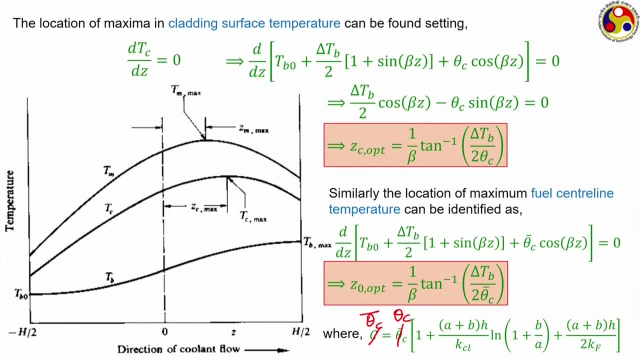 profiles. if you want, we can also calculate the optimum location for the temperature, where the temperature is maximum at the fuel cladding interface. but generally that is not of a great interest, or major interest is to know where the fuel center line temperature is maximum. that we can obtain here. 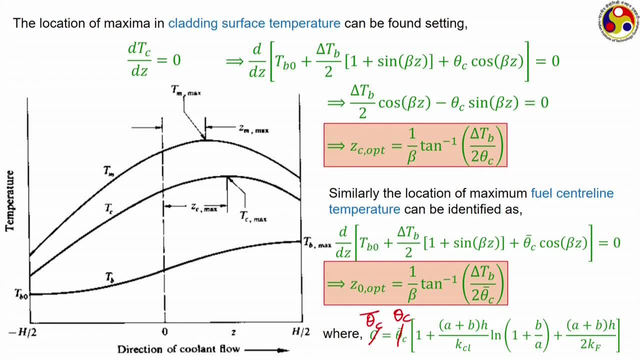 And by putting these expressions for z optima in the corresponding temperature expression you can also get the value of this: maximum temperatures like the maximum cladding surface temperature or maximum fuel center line temperature or maximum temperature value at the interface of the fuel and cladding. but those generally are quite big expressions. that is why they. 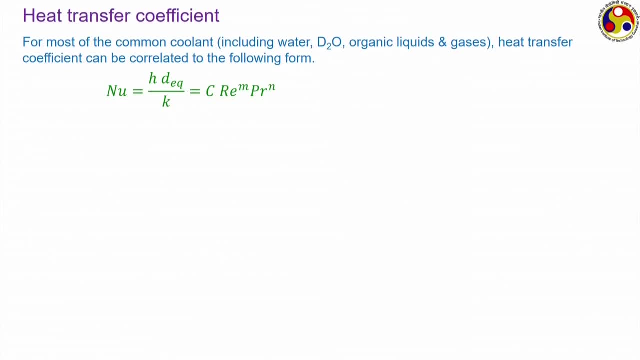 have been avoided here. Next, we need to know about the heat transfer coefficient. We know that the generally, there are three, three resistances that we have seen. One important thing is that the analysis that we have just done, while the concept of fuel, thermal, the thermal resistances were developed following 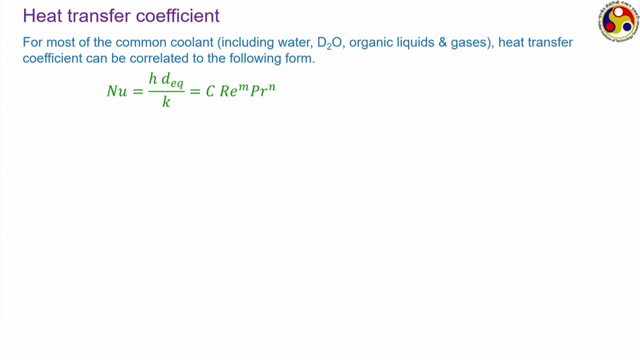 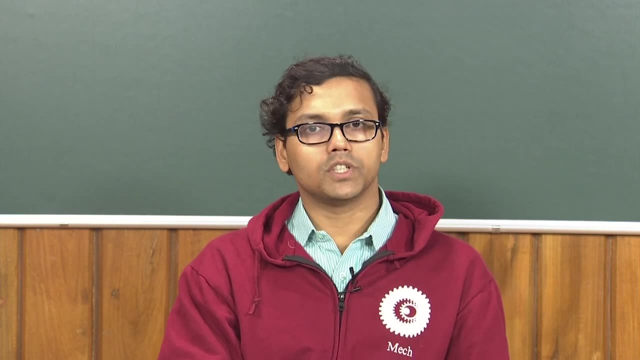 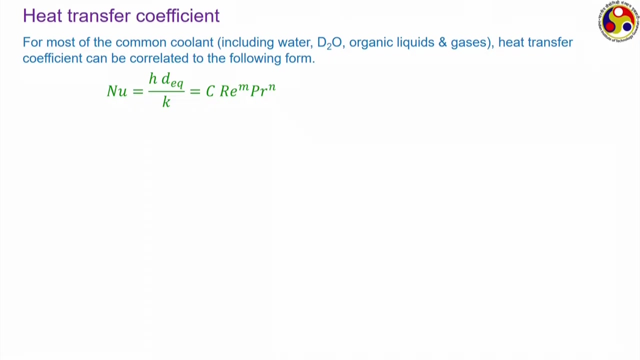 an uniform heat transfer distribution or uniform value of the heat generation throughout the reactor. But when we are having some kind of distribution for the heat generation in the radial and axial direction, both we can still use the concept of those resistances, And two of them being conductive resistances. they are very standard because a thermal once 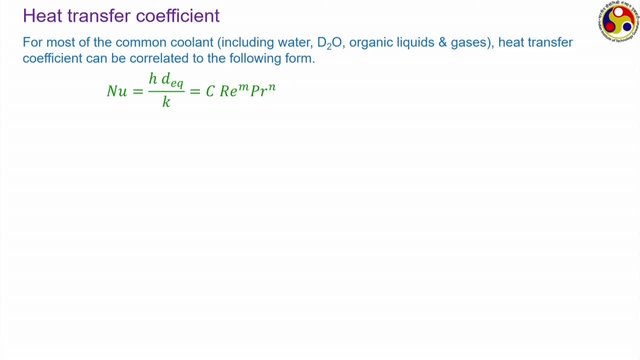 we have selected the material, we know its thermal conductivity and corresponding resistances values. as once we fix up the dimensions as well, corresponding resistance values are fixed. But the convective resistance depends on the heat transfer coefficient, And the heat transfer coefficient may depends on infinite number of factors, like it may depend on what is nature. 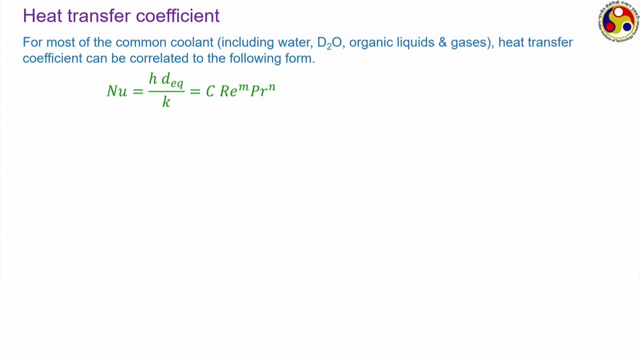 of the coolant. what is the nature of the cladding outer surface, that is, a surface where the solid and fluid are having some kind of interaction. what is the nature of the flow itself, whether it is laminar or turbulent, and similarly, several other factors. 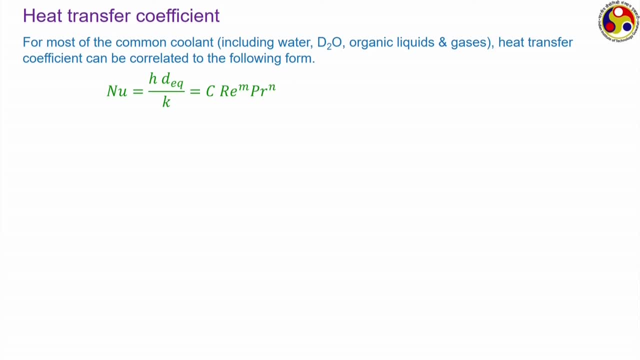 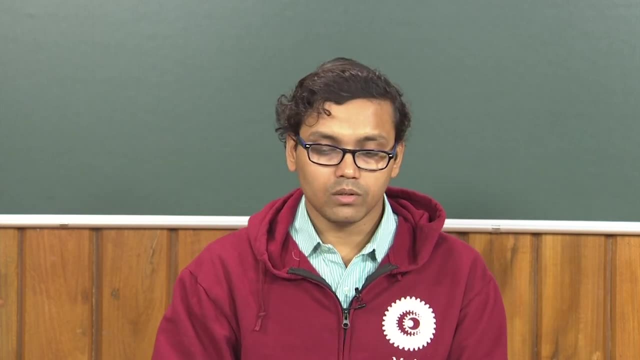 But commonly for any general coolant like water or heavy water or organic liquids or gaseous, heat transfer coefficient can have a form like this: A Nusselt number can always be expressed as a function of Reynolds and Prandtl numbers. Here Reynolds number is defined. 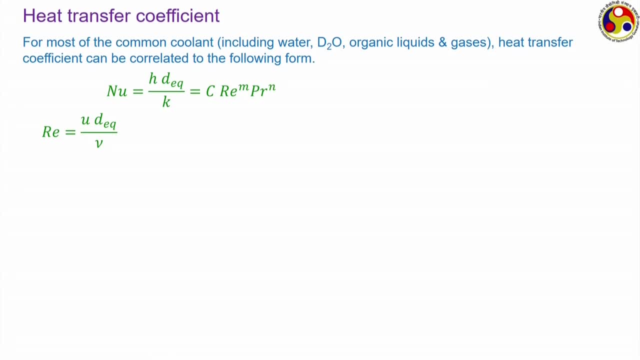 as form like this: Similarly, here, u is the velocity of the coolant and nu is the kinematic viscosity of that, which is generally corresponding to the average temperatures. And other term that we can find in the definition of both Reynolds number and Nusselt number is D equivalent. 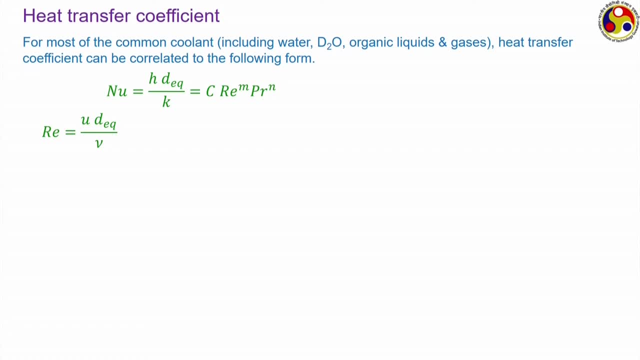 which actually is a suitable length scale, And it is also called the equivalent diameter, D equivalent it is, or hydraulic diameter also is a much very common name. Now, equivalent diameter has a definition of 4 AC by pi, where AC is the corresponding cross diameter. So 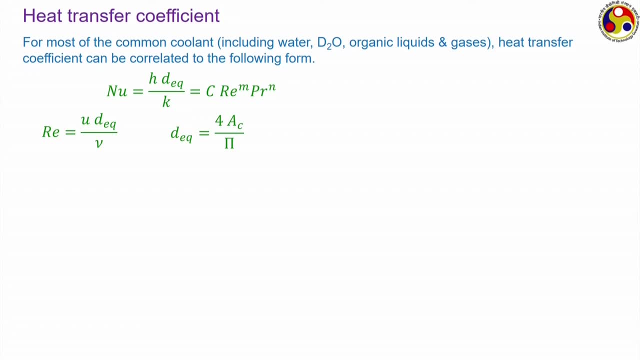 cross section area and pi is the weighted perimeter. Now if we are dealing with a channel with circular cross section- say your geometry is that of a circular channel and through which the coolant is flowing, then calculation of this D equivalent is very easy. This case, if D is the diameter of this one, then D equivalent. 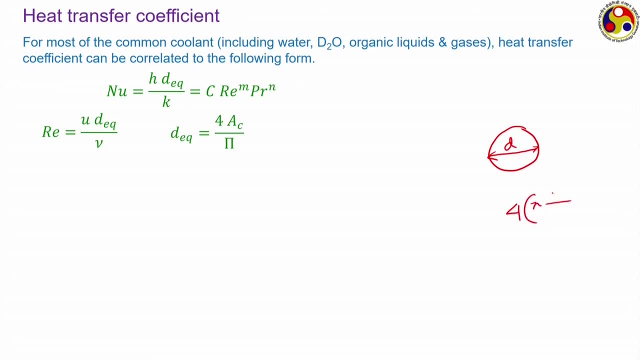 is 4 into the area of this one area should be pi D square by 4 and divided by what should be the weighted perimeter for this. This is pi into D, So it comes equal to D. That is when you are having dealing with a circular channel. 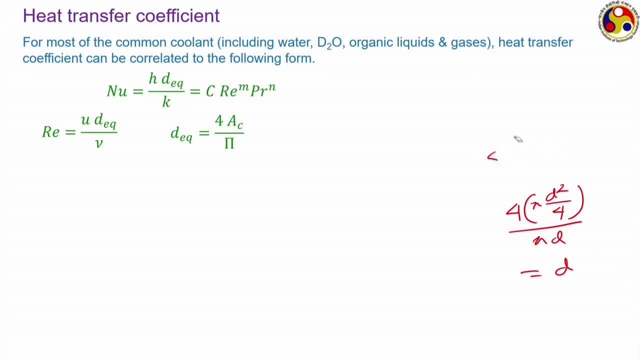 this is just reducing to the diameter of the channel, But when you are dealing with a non circular duct channel, then we have to find a way of calculating this. D equilibrium Like this one is the common representation of fuel and fuel rods and coolants inside the reactor. 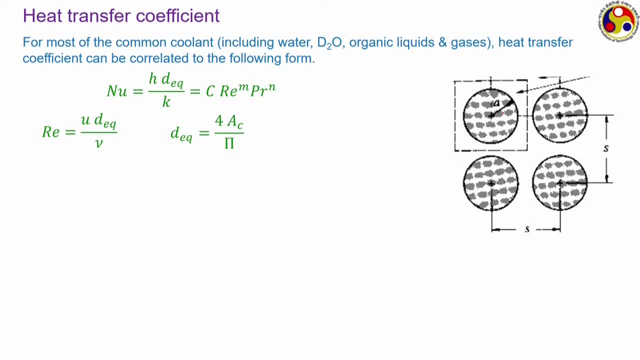 Here we are having circular fuel rods, each of radius a, And we can select a square of size S around each of this. Here S is the spacing between successive fuel rods. So this, this particular portion, this hash portion, can be viewed to. 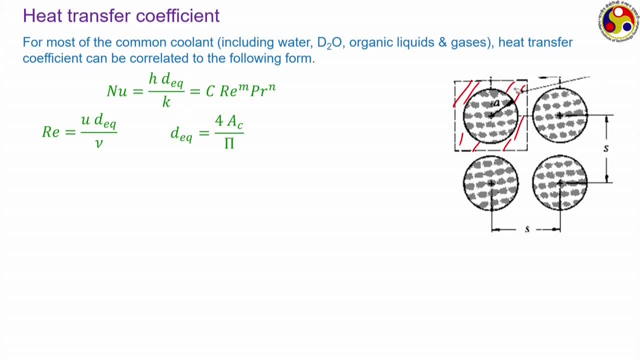 be occupied by the coolant, Like we have done. we have considered earlier in our earlier analysis. In this particular case we can calculate equilibrium dimension to be something like this: So the area for each such S square is the area of the square and the area occupied by 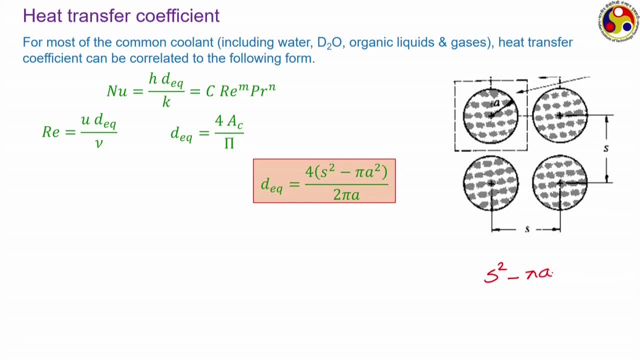 the coolant will be this minus the area of corresponding circular fuel rod. So this pi S square, this multiplied by the 4. And what is the corresponding weighted area That has to be the perimeter of this particular circle or circular fuel rod, which is 2 pi. 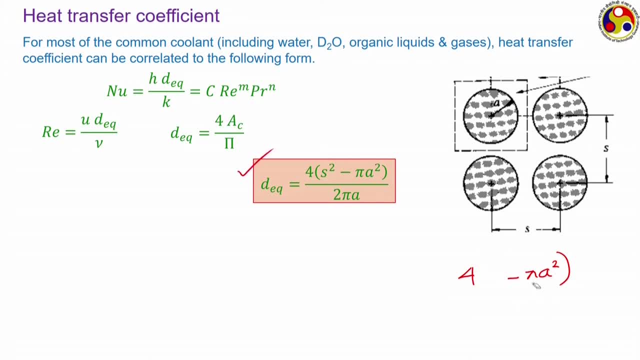 a. That is precisely what is written here. So this is your. this is the most common geometry, but if the geometry is something else, we can the same way calculate corresponding equilibrium lengths, equivalent diameter or the length scale. to identify Reynolds number and Nusselt number, There are several ways. 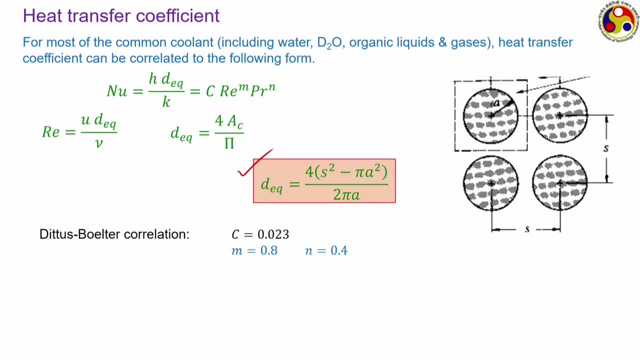 we can put the values of this coefficient, C, and these two exponents, m and n. One can be the age old details goiter correlation, where C is 0.023,, m equal to 0.8 and, this being a heating case, n equal to 0.4.. But there are several others experimental relations. 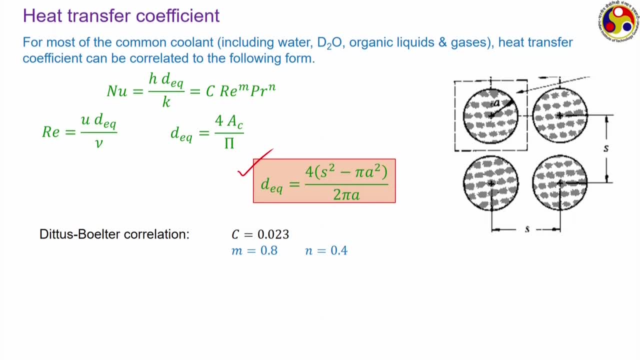 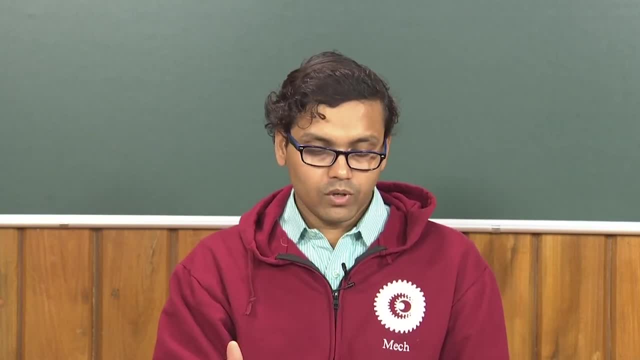 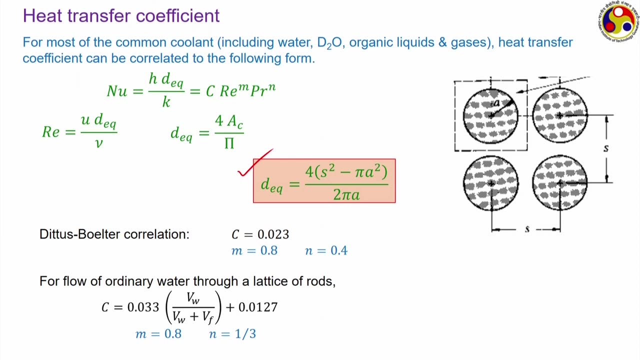 Here we have to depend upon experimental correlations to identify the expression for Nusselt number For ordinary flow, for flow of ordinary water through a lattice of rods. this is one correlation that that sometimes is used in nuclear thermal hydraulics. Here you can see: m equal remains the same, that is, 0.8, and n equal to one-third, but C is 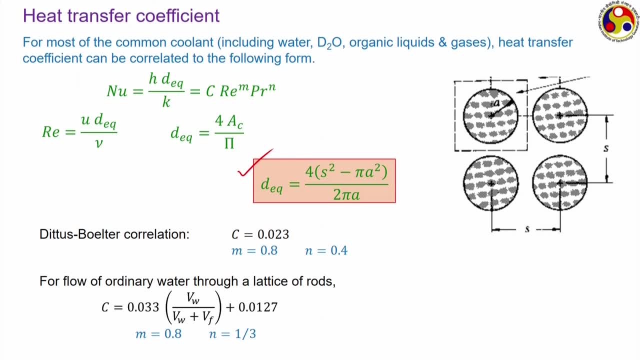 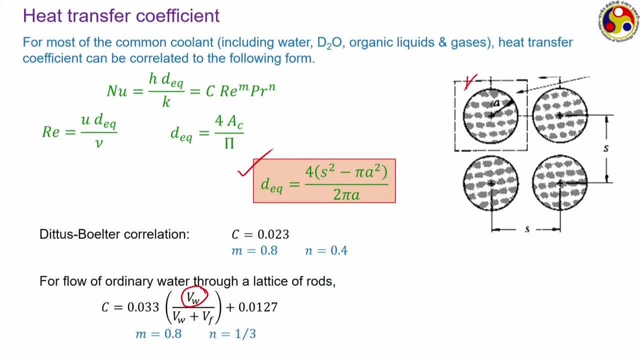 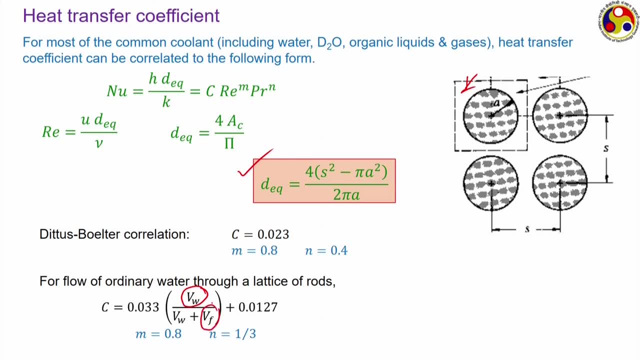 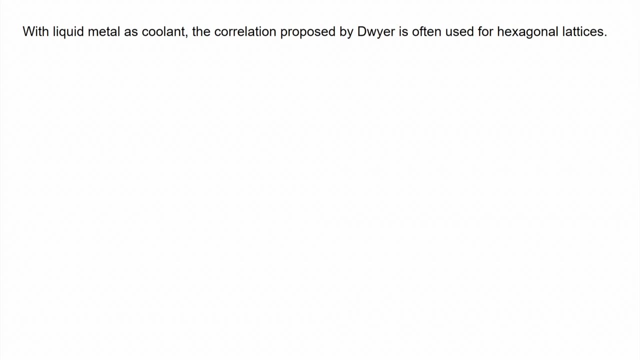 And this is V f, the volume of fuel, the fuel rod corresponding to, again such, each selected volume. There can be several other correlations as well which are applicable for such kind of coolants And if we are using liquid metal coolant. liquid metals have much higher thermal conductivity compare to the other thevan. 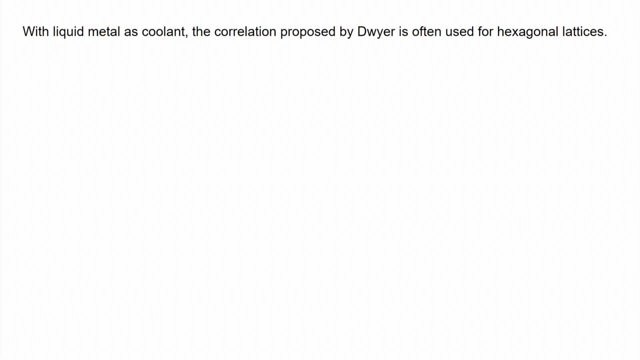 other coolants and therefore those are detached boulder kind of relations are not applicable. One correlation that is commonly used in those proposed by Deweyerparticularly for hexagonal lattices is like this: Here S is the same, that is, a spacing between neighboring fuel. 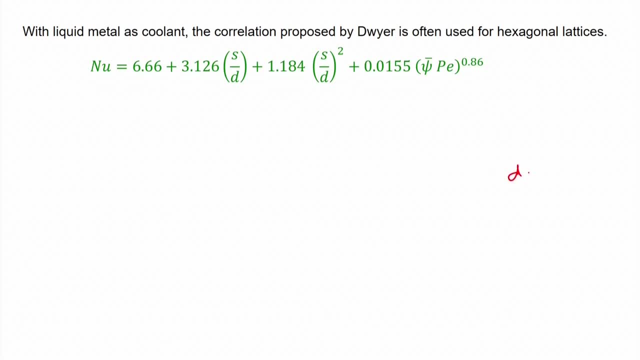 rods and the D is the diameter of the fuel rod. So D is actually twice of this A. This psi bar is some kind of empirically fitted constant where we can find Prandtl number and Reynolds numbers involved, and also you have Peclet number P, which is the product. 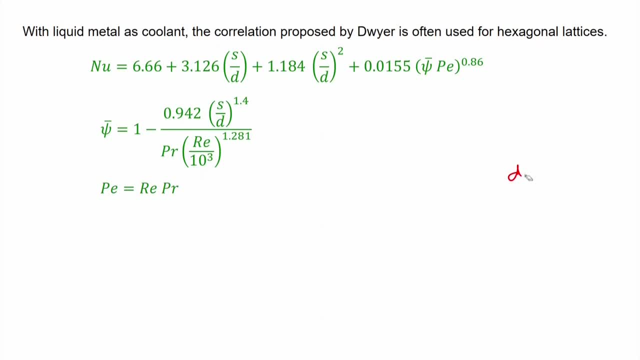 of Reynolds and Prandtl number. So this is one correlation that can be used when you are having liquid metal as the coolant, but this one has a restriction: this is applicable only for S greater than 1.35 times the diameter, And if we are dealing with a channel where 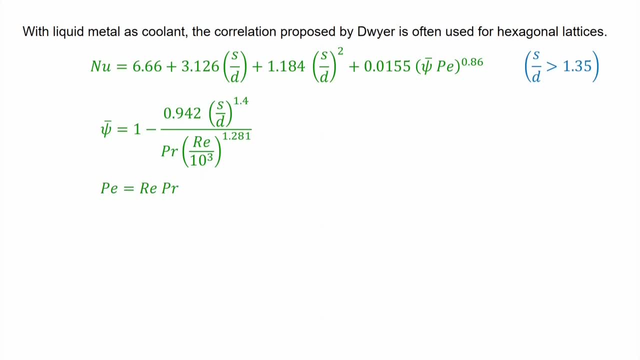 the diameter is less than 1.35 times the diameter, So the diameter is much, or this S by D ratio is much smaller- a much tightly packed lattice. this can be one of the relations that can be used If we are using a lattice which is 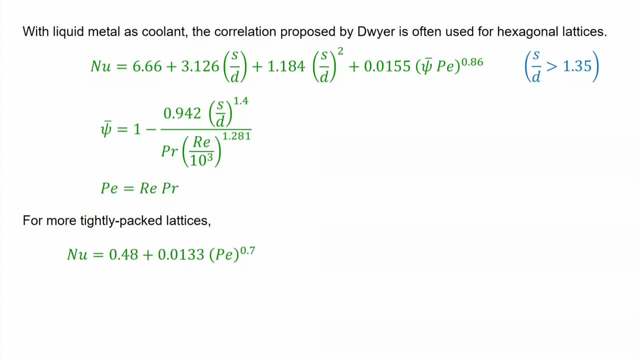 not hexagonal in nature, some kind of a, say, triangular lattice or a square lattice, then this Nusselt number relation can be multiplied with a suitable conversion factor and then the same formula can be used. So this is the typical nature of the temperature distribution that we get across the liquid. 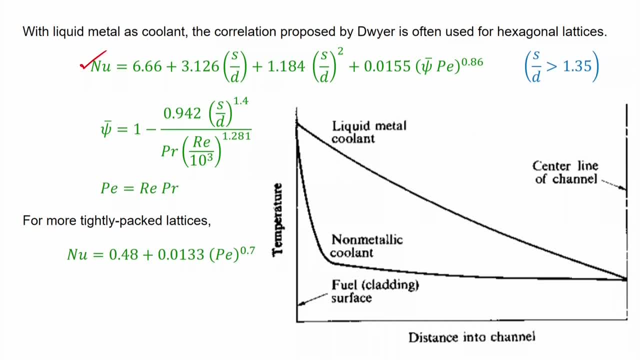 flame. When you are having a non nonmetallic coolant, there you can. the thermal conductivity being small, corresponding resistance is quite large and we can see this is rapid reduction in the coolant temperature quite close to the surface. But if we are using liquid coolant or liquid metal as the coolant, because of high thermal conductivity it increases quite 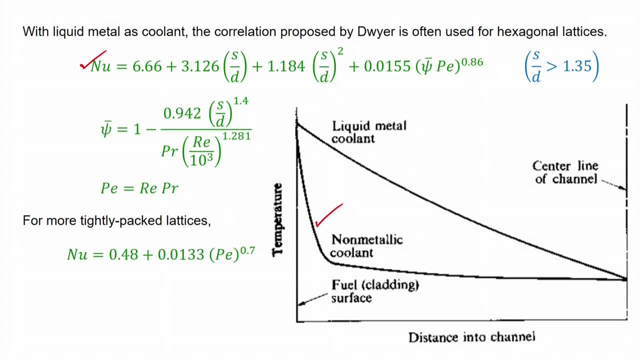 gradually And almost following a straight-line kind of validation. but this is applicable. this relations are applicable when we are dealing with single phase coolant. But there may be several situations, particularly in boiling water reactors, where actually there is a phase change involved in, say, the reactor that is. 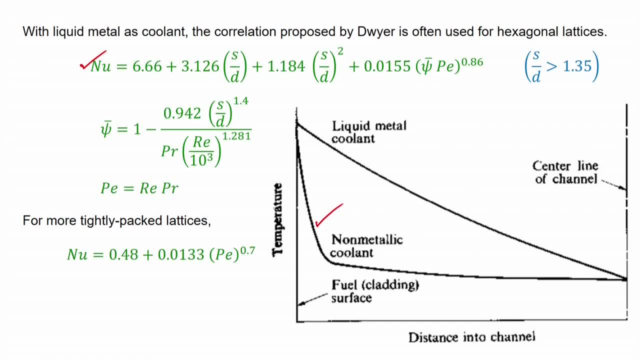 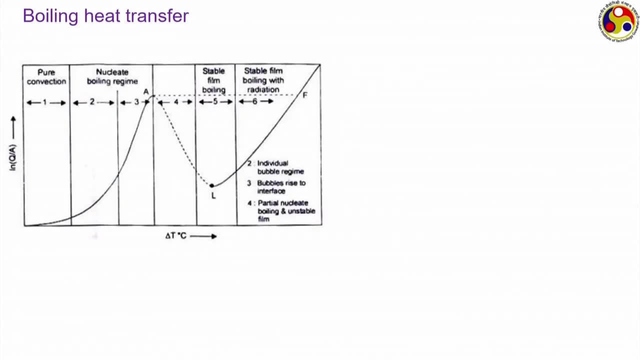 liquid coolant, like liquid water, enters the channel. there, after absorbing heat, it reaches the corresponding saturation temperature And then again it can start to get converted to vapour phase. So in such kind of situation we need some knowledge of boiling heat transfer. I hope all of you have idea about this and this, as this is the classical diagram available. 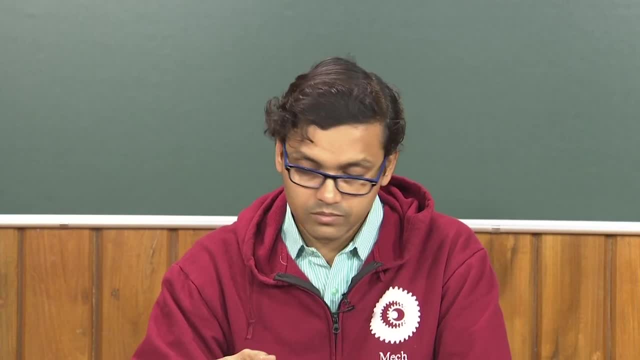 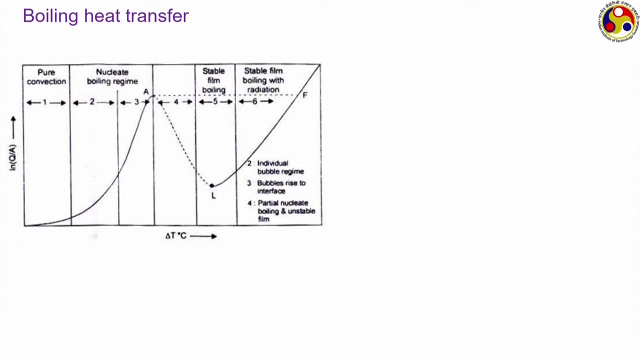 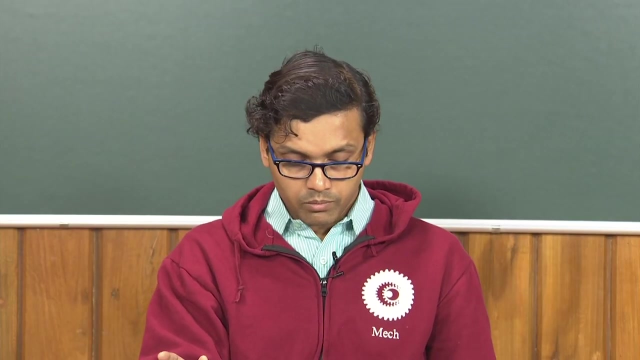 in almost every heat transfer book but just for the purpose of completion, the completeness of this one, I am mentioning here about the boiling curve that we may get for pool boiling situation. Pool boiling refers to where we are heating up a some quantity of fluid in. 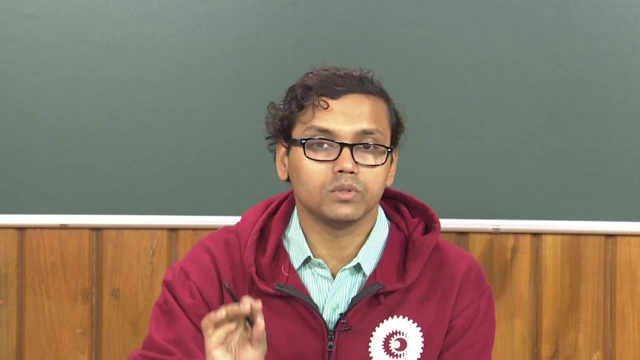 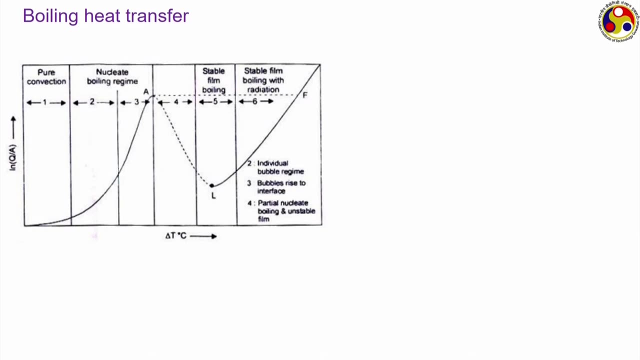 an open container So that there is no exclusive flow before the initiation of heat transfer. In such kind of case we get 4 clear regimes of heat transfer here: on the horizontals- sorry, the vertical axis- the heat flux is plotted on logarithmic scale and in the horizontal. 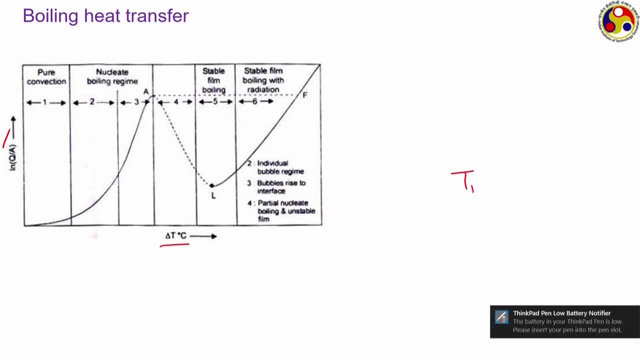 axis We have delta T, which is actually the wall temperature, minus saturation temperature corresponding to the pressure at which this experiment is being conducted. So initially we get a pure convection zone where liquid is present, pure single phase liquid, and phase change is yet to get started. Then we enter a nuclear boiling regime where we have isolated bubble formation. 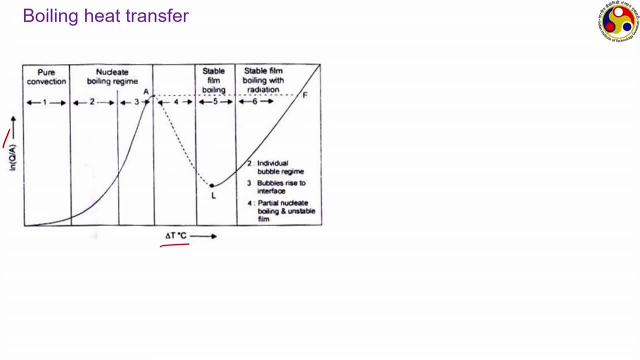 at the heating heated surface. We have aっていう point which after some time may get detached from the surface and then rise because of from the buoyancy effect, Then something not marked here. this is an intermediate zone where it is difficult to say exactly what is happening. and then we 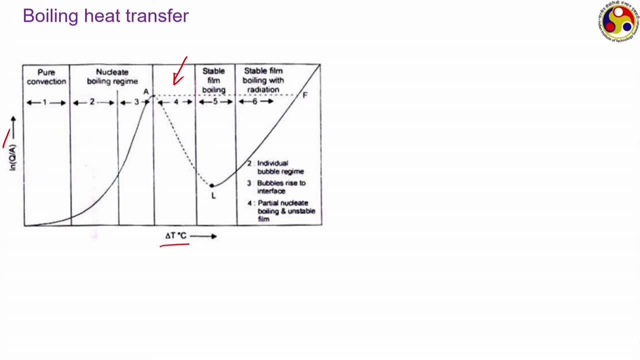 have a stable film boiling zone where a film of liquid, or I should say film of vapor, is formed on the heated surface. This intermediate zone can have characteristics ofboth nucleate and flim boiling. This particular point corresponds to the maxima in the anyways in which the pressure 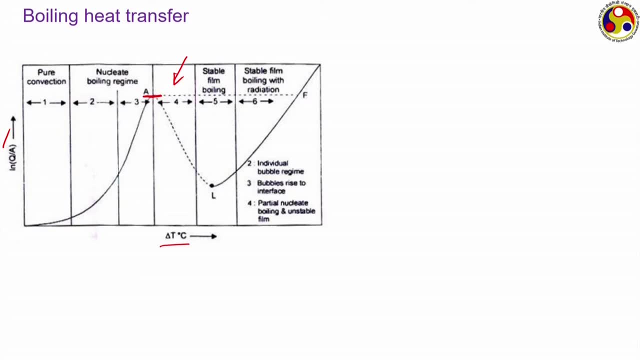 and flow of liquid and pressure are distinct. So this is the very important point, which is in the, the maximum heat flux corresponding to a nucleate boiling regime, and it is hence called a critical heat flux. If we are dealing with the water and atmospheric condition, this 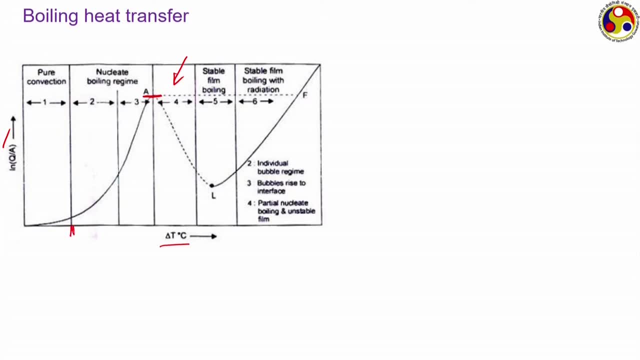 pure convective zoneruns up to 5 to 6 degrees of this delta T, whereas this critical heat flux typically appears aroundaround degree of superheat of 30 degree Celsius And the corresponding heat flux value corresponding to critical heat flux can also be high. it. 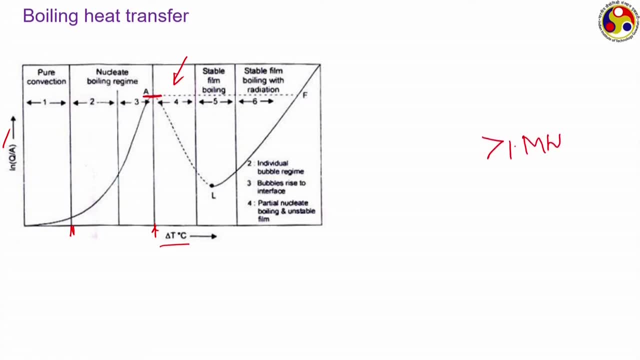 is invariably greater than 1 megawatt or 10 to the power, 6 watt per meter square, because this is heat flux that we are talking about. But this applies to pool boiling and the situation that we are having here. that is not pool boiling, rather that is flow boiling situation. as the 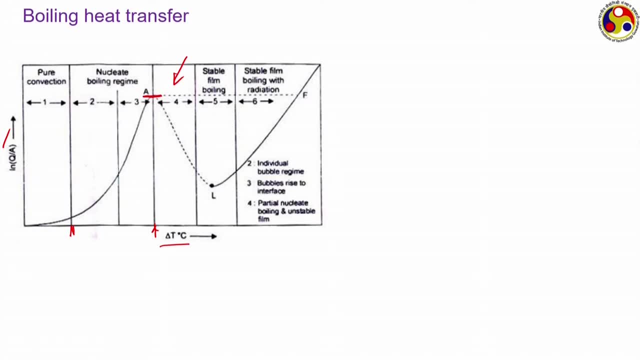 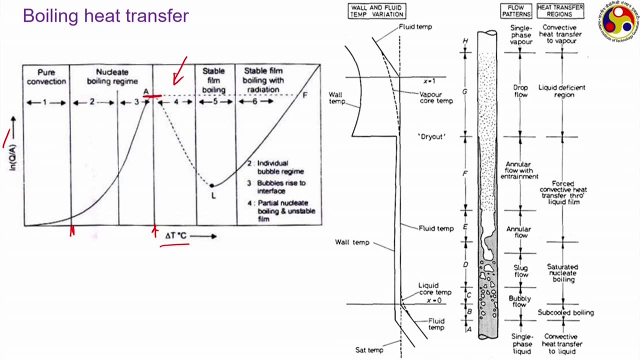 liquid is flowing as it is entering the channel. So in that kind of situation- this again a classical diagram- here a liquid is flowing upwards through a heated channel, So it enters as a single phase liquid here andcontinues to remain a single phase: liquid till location. 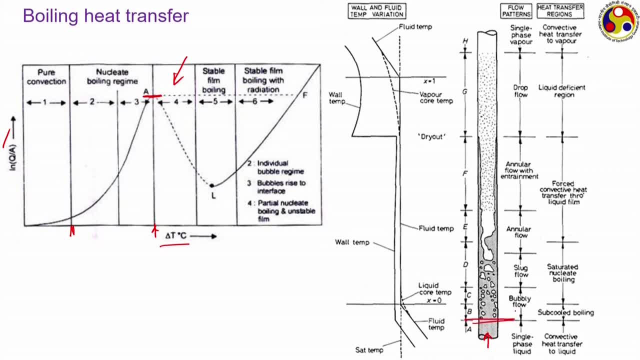 somewhere here Where we can see small bubble that may generally gets formed at the surface and as we keeps on moving upwards, those bubbles keep on increasing in size and then they starts getting separated from the walls. As we move further, the smaller bubbles generally agglomerate together to form bigger bubbles and in case of bigger, bigger bubbles, they 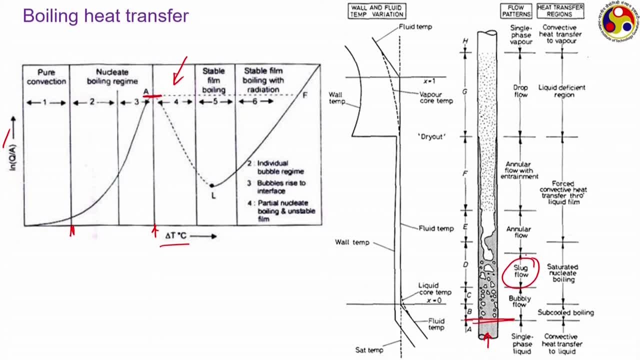 will start to form bigger bubbles, And then they will start to form bigger bubbles, and then they will start to form bigger bubbles, and then they will start to form bigger bubbles. We get the slug flow regimeand the corresponding bubbles are called slug bubbles or Taylor. 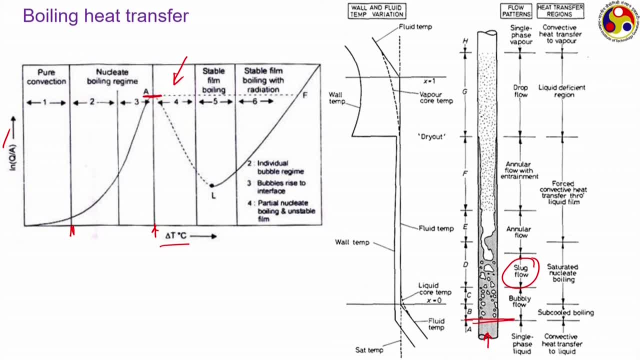 bubbles. Thesebubbles are generally of a bullet shaped, that is, around, having a rounded head and quite flat on the rear side. As we move further down, this bubbly flow gives out to the annular flow regime. In the annular flow regime we haveliquid restricted only to 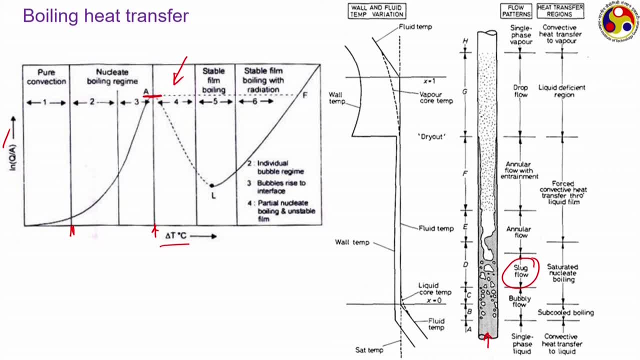 the wall and the vapor occupying most of the slug. So this is the center part of this, of this heated channel, and this way it keeps on going. in practical reactors we generally do not go up to the annular flow regime or may reach quite close to that, but we generally do not want to go even beyond where the entire liquid 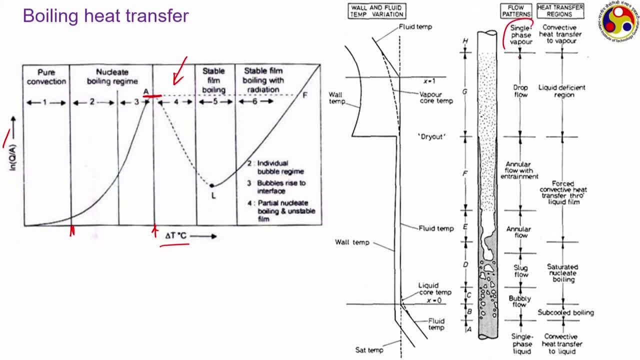 gets converted to vapor and we are dealing with something like a single phase vapor zone Corresponding heat transfer variation or the wall and fluid temperature variations are shown alongside. Where we are dealing with a single phase vapor zone, The surface temperature thatkeeps on increasing till some point here, or I should say the surface. 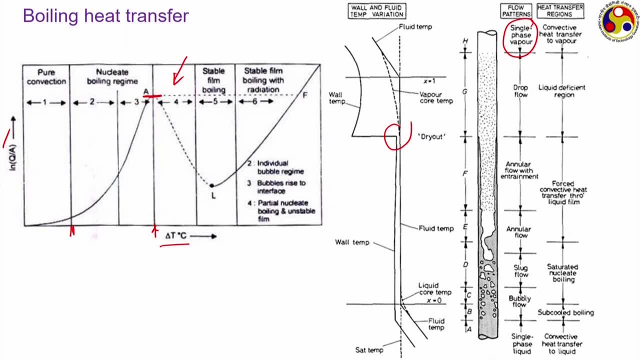 temperature initially increases and once thesmall bubble starts to appear somewhere here the surface tension, The corresponding wall and fluid temperature variation is shown here. Initially both the temperature keeps on increasing almost in proportion till small bubble starts to appearsomewhere. here the small bubble starts to appear. 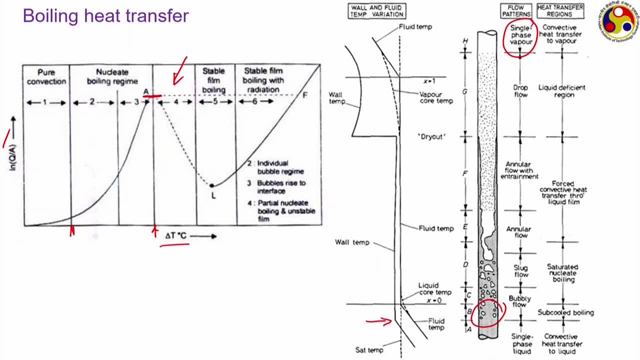 But interestingly, in this zone the fluid temperature is yet to reach the saturation and that is why they are often called the sub cooled boiling zone. Sub cooled boiling is is a situation where the walls are at a temperature higher than the saturation, and that is why small bubbles may starts appearing at the walls. 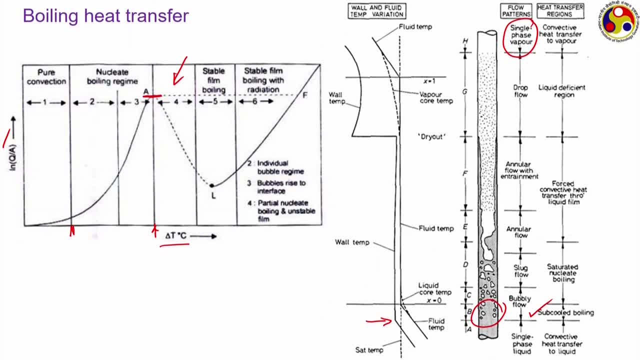 Butas, soon as those bubbles get separated from the walls, they come in contact with highly sub cooled liquid and therefore they gets condensed. As the temperature of thebulk fluid keeps on increasing and is about to reach the saturation, then some of the sub cooled bubbles may survive in the bulk of the liquid as well. 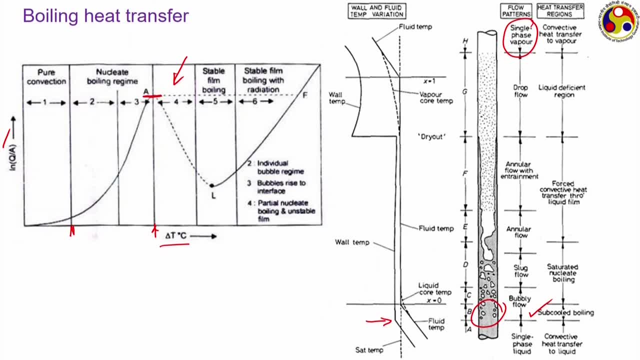 But once the bulk of the liquid reaches saturation, then we call that saturated boiling. So once we enters the saturated boiling zone, then the wall temperature remains constant and the fluid temperature also remains constant at the saturation temperature. This entire portion is called the nucleate boiling zone, which is analogous to the saturated boiling. 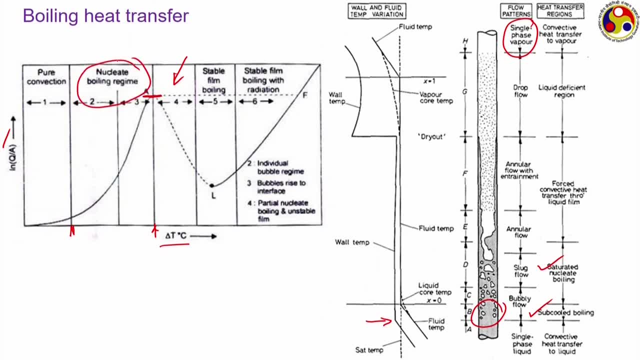 zone. So that is why the bulk of the liquid keeps on increasing and is about to reach the saturation to this nucleate boiling regime of pool boiling. But this saturatednucleate boiling continues till the appearance of the annular flow regime, where we have the force convective transfer, and finally the liquid deficient zone, where 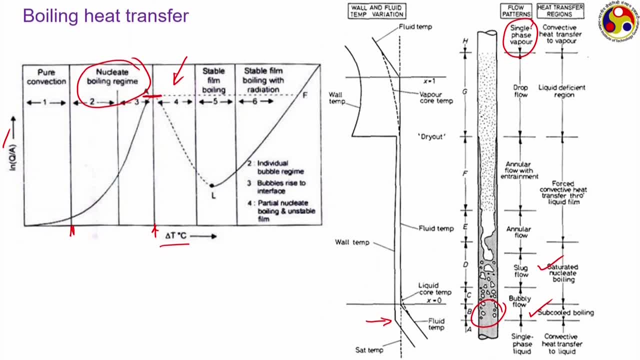 the film on the wall that completely evaporates. And when, at this particular juncture, when the liquid film at the wall completely evaporates, then theheat that is supplied to the wall it has nowhere to go, basically Because there is no liquid film in contact with the wall. 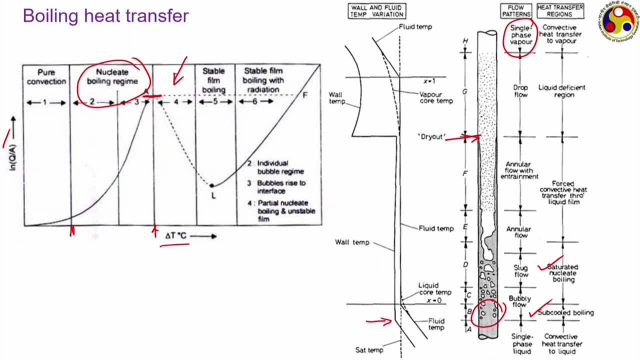 there are onlyvapor, which is having a very poor conductivity, and maybe some small liquid droplets, whichyou can find here in these, which are just floating around in the vapor and they are not likely to come in contact with the wall And therefore there is a suddendecrease. 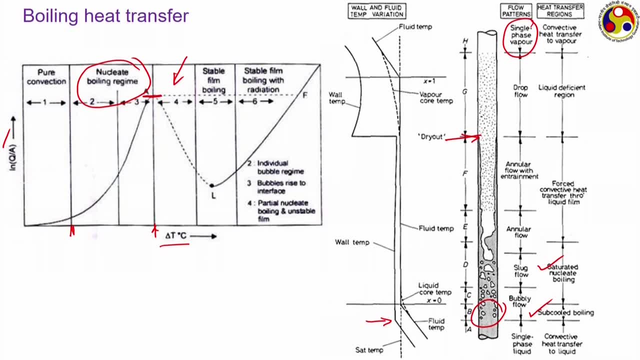 in the communication between the heat transfer, communication between the wall and the fluid, which is referred as the dry out. So in the dry out zone you can clearly see that the temperature of the wall suddenly jumps to a very high value and this difference can be quite significant. Fluid temperature continues to be the saturation temperature till all. 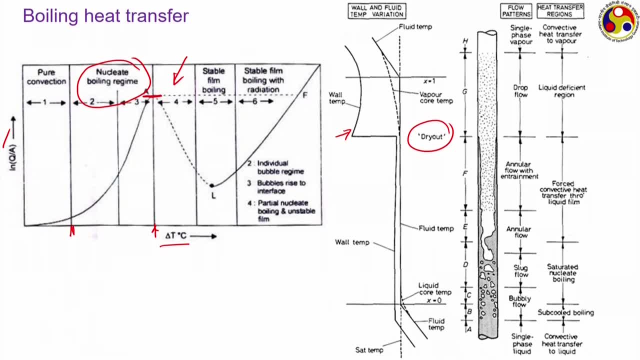 this liquid droplets completely evaporates and then, once it reaches a perfect vapor situation, then only it starts to increase. This entire topic of boilingheat transfer, or this flow and pool boiling, is extremely complicated and requires, I should say, several lectures. So for this, but as our purpose is only to get an idea about the nuclear thermal hydronics, 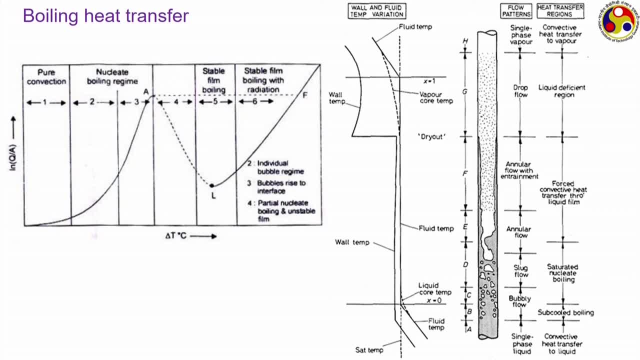 So just to know the names of all these regimes is sufficient. So we can see that in a typical coolant flow through a channel, in something like in a boiling water reactor, we get different regimes, like initially a single phase liquid regime, then a sub cooled boiling regime. 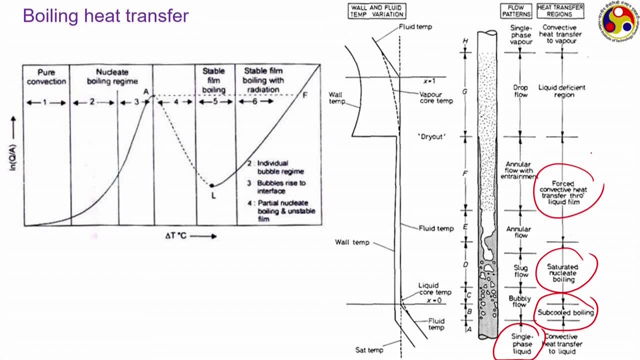 then saturated nuclear boiling regime, a forced convective heat transfer regime and finally liquid deficient regime going to the convective heat transfer to single phase vapor. And in terms of the flow regimes- that is the visual nature of the flow regimes- we may have a bubbly flow, then we may have a slug flow and giving to annular flow and finally a drop. 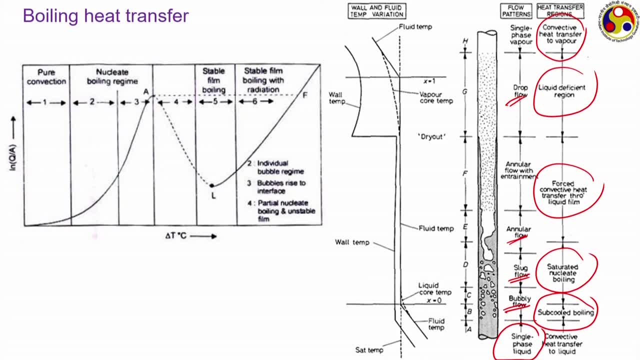 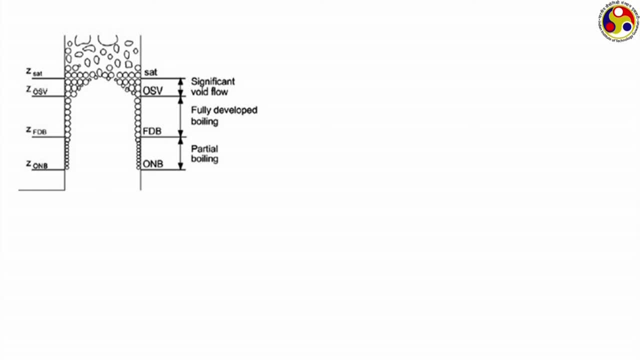 flow regime where we are only having liquid drops floating in vapor phase. If we look further into the sub cooled boiling part, till some point which is called ONB, that is onset of nuclear boiling. So the Blessing LUT is a completely separate and a cross exposed on face vapor at which 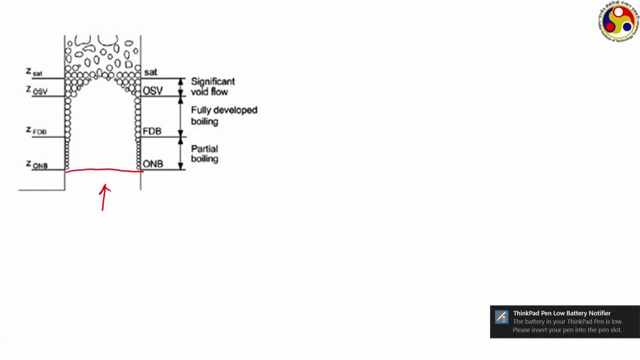 we know there is also isonly single phase vapor, something like this. Here the flow is considered fromsomewhere downstream location in the upward direction, But ONB 2, something called FDB, the fully developed boiling, there are only very minor, almost ah, microscopic level. ah vapor bubbles can be identified in the walls as we reach this fully developed. 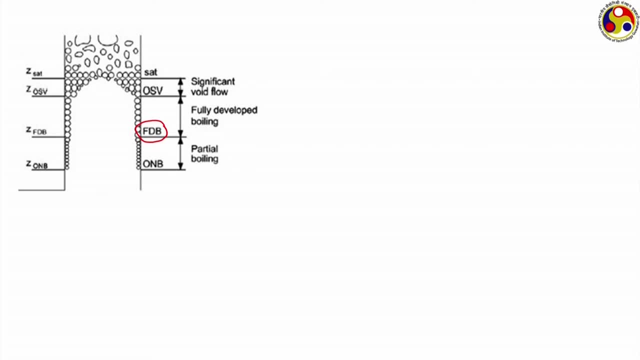 boiling zone, the temperature difference between wall and saturation, temperaturedifference between the saturation temperature It will affect in a to be We called as stochastic vapor, vapor, vapor temperature and the bulk fluid temperature is much smaller. So much bigger bubbles can be seen on the walls, but still there are no vapor bubbles in the bulk of the fluid. 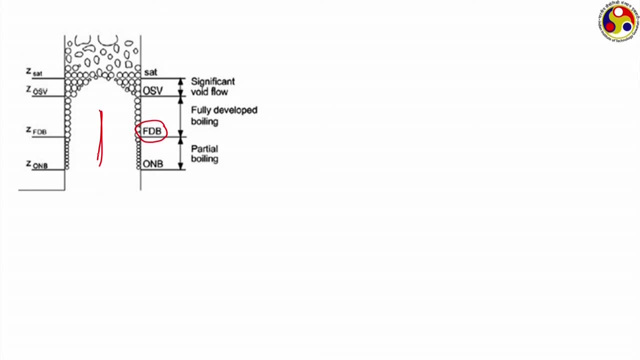 because in the bulk in this close to the center line, the temperature is way below the saturation. Then we reach something called OSV, onset of significant void. This is the location from where the bubbles can actually get, can actually survive, even after getting detached from the. 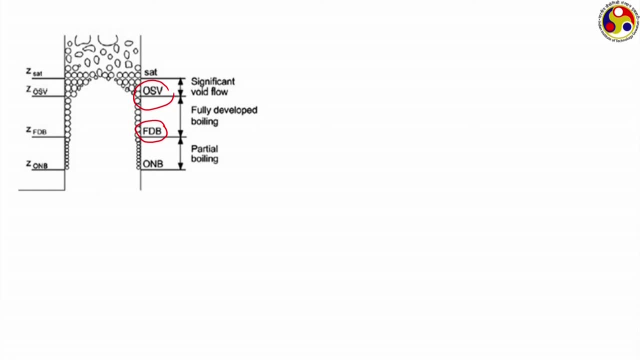 wall, because here the degree of sub cooling for the liquid is quite small and very soon the entire fluid reaches the saturation temperature. So the mechanism of sub cooled boiling is quite, very much different compared to what we have in case of saturated boiling, because saturated boiling the entire fluid is already. 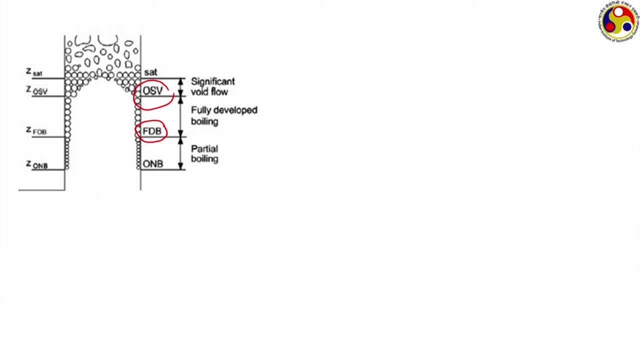 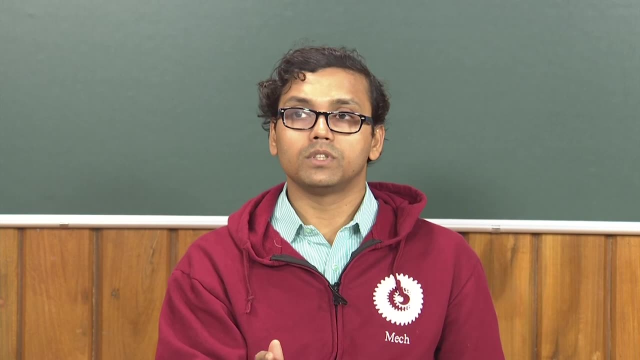 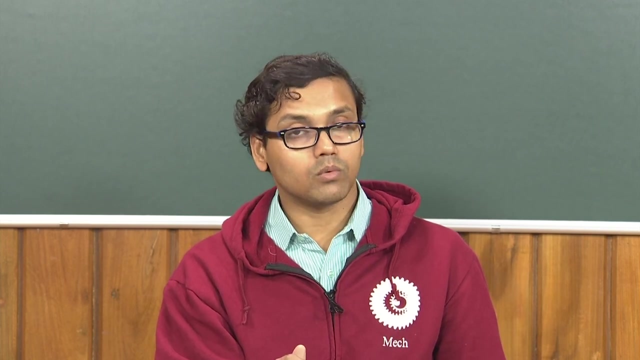 in the saturation temperature And so whatever heat that is supplied, that entirely spent to ah, entirely spent to vaporize the fluid is entire heat contributes as latent heat. However, in the subcooled boiling zone a part is utilized as latent heat to produce vapor at the walls, but a major part is utilized. 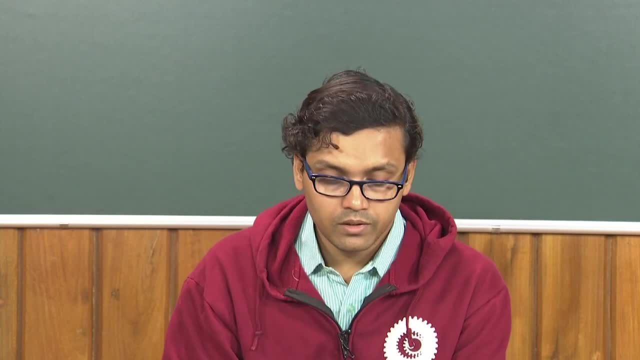 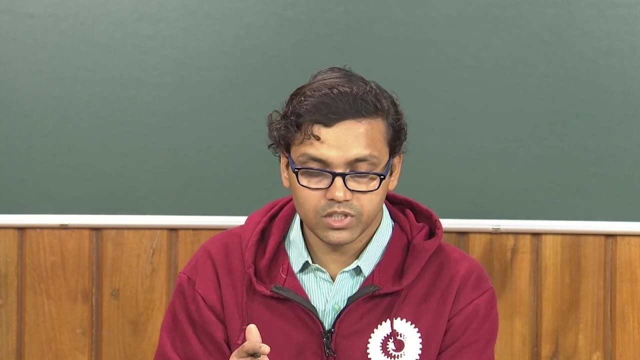 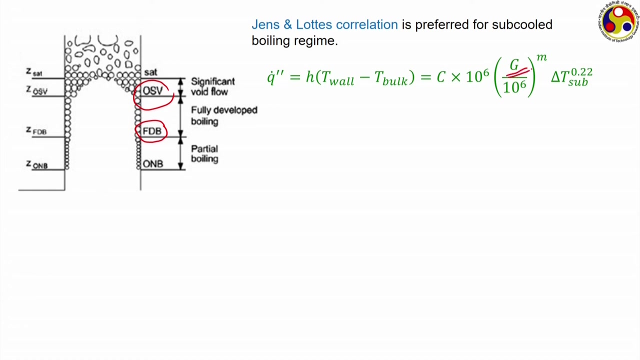 in heating the single phase liquid And accordingly we need to use different kind of heat transfer correlations for subcooled boiling zone and the saturated boiling zone. For subcooled boiling zone, the Jensen-Lauter correlation is preferred, which is having a form like this: Here, this G is the mass flask, which is basically the mass flow rate divided. 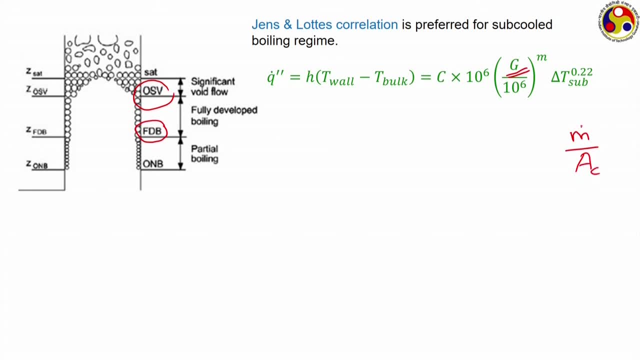 by cross section area of the channel, mass flow rate of the coolant by the cross section area And delta T sub is the degree of subcooling at that particular location. delta T sub, as I have mentioned, it is just saturation temperature minus bulk fluid temperature. M and H is the 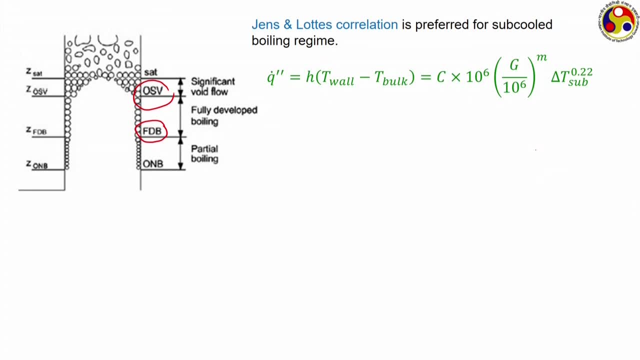 heat transfer coefficient. M and H is the heat transfer coefficient. M and H is the heat transfer coefficient, And C are two coefficients which depends on the local pressure. and these are some representative values Once you reach the saturated boiling zone, particularly in smooth circular tubes, 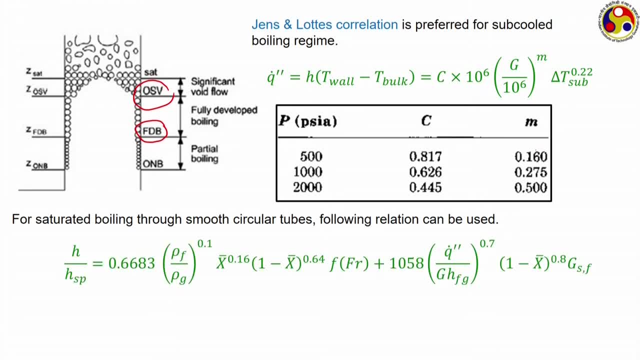 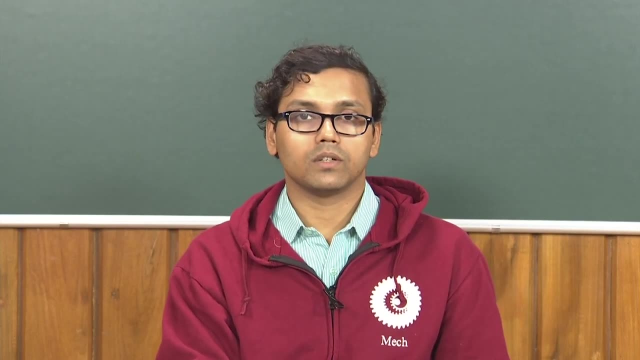 this is one relation that can be used. You can see, it is a quite complicated form. actually, There are several such correlations exist because this is an active area of experimental research And it has been found that this heat transfer correlations can be divided into two phases, And if this is half phase, then the heat transfer coefficient can depend. 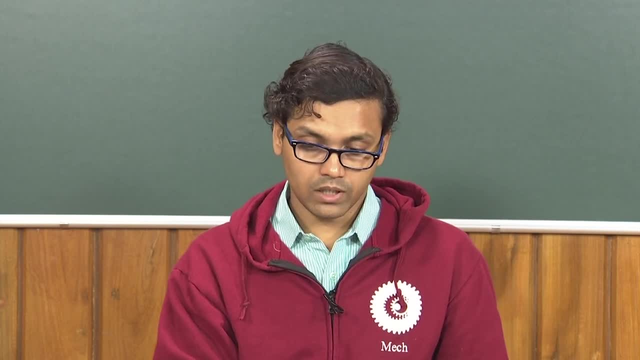 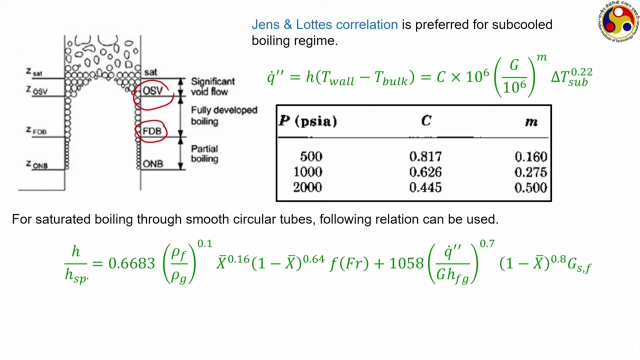 on infinite number of factors when two phase flow is involved. This is just a representative one to give you an idea how complicated it can be. You can see on the left hand side we have H upon H single phase. Here H sp refers to the single phase heat transfer coefficient means, instead of being a two phase mixture. 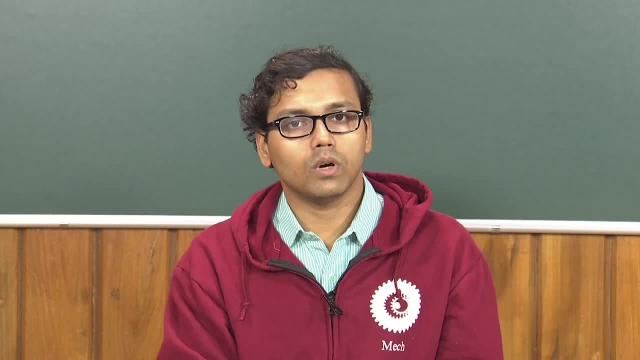 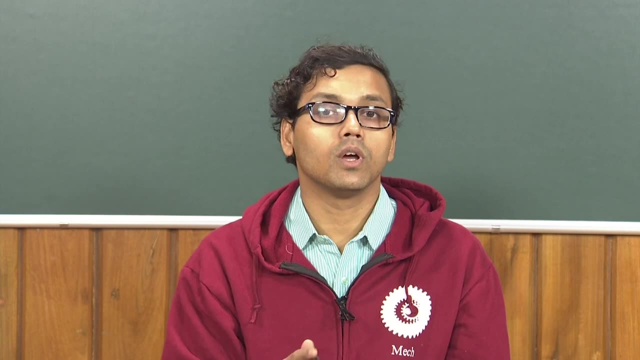 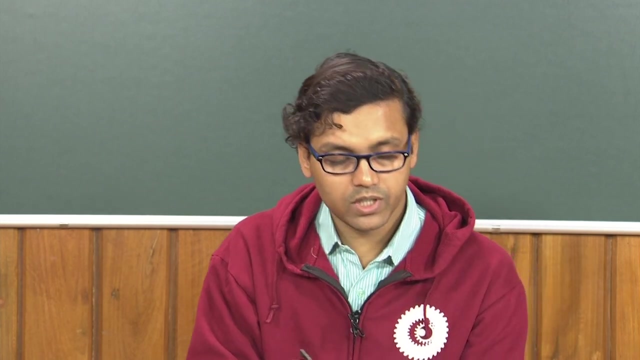 if the entire fluid is flowing as a single phase liquid, then what would have been the corresponding heat transfer coefficient? And these H sp is can be calculated using something like Dittus-Volta relation, or maybe the one that I have referred earlier On the right hand side. first we have the density ratio. here rho f is the saturated liquid density. 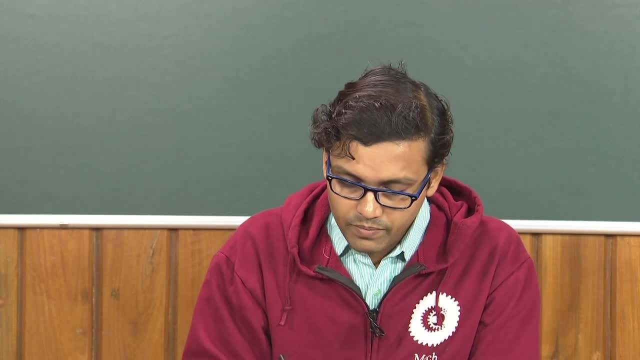 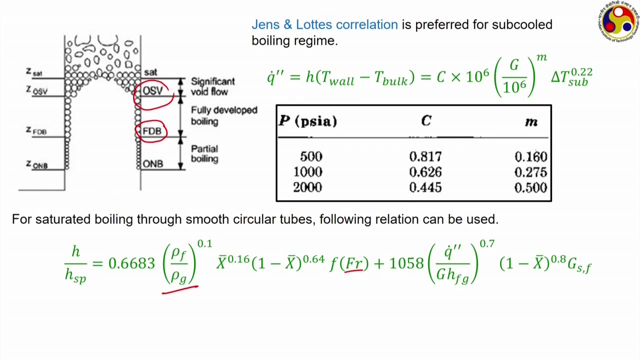 and rho. g is the saturated vapor density, f, r is the Froude number. A Froude number is not a non-dimensional number which present the ratio of inertial and gravitational forces, And Froude number typically is defined as root over u, square by g into L where u is. 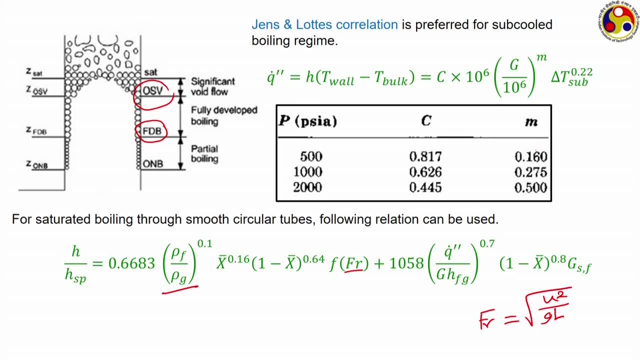 the velocity of the fluid, g is the gravitational force and L is some suitable length scale, Like if we are talking about flow through a smooth circular tube, then L can be the diameter of the tube, So it it is u by root over g into D in that kind of situation And this: 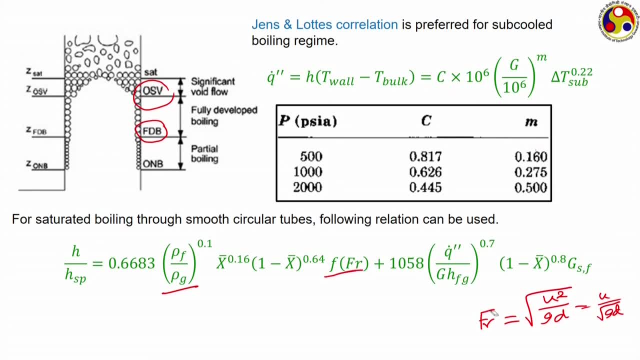 function And f function of Froude number. this actually depends on the exact orientation of the flow, that is, we are having an upward flow or downward flow, maybe some idea about the surface roughness, etcetera. Then we have: this is the heat flux that is applied to the wall. h, fd is the latent. 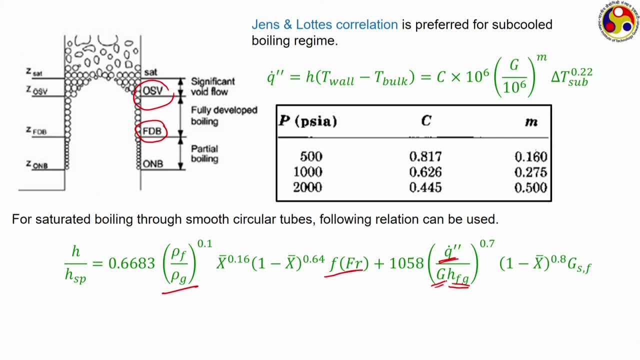 heat of vaporization, and g is the mass flux, which I have just mentioned. And finally, there is another, gs, which is actually a coefficient which depends on the combination of the metal that is used in the surface and the fluid itself. And x bar is the mean vapor mass fraction, which is defined like: this is the area averaged. 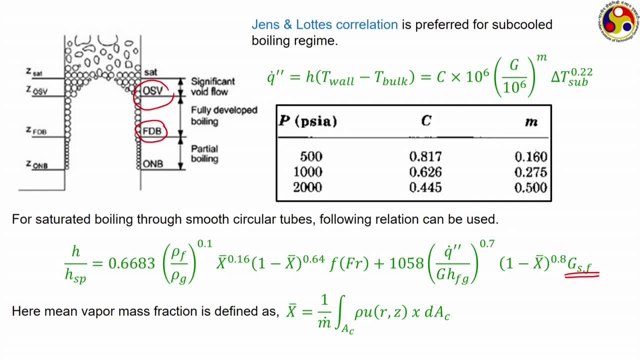 mean for mass fraction, because in a single cross section there may be significant different in the mass fraction value, Like if we take a sample somewhere here at at this particular cross section. at here you will be getting some value of the vapor cross section. vapor void fraction. 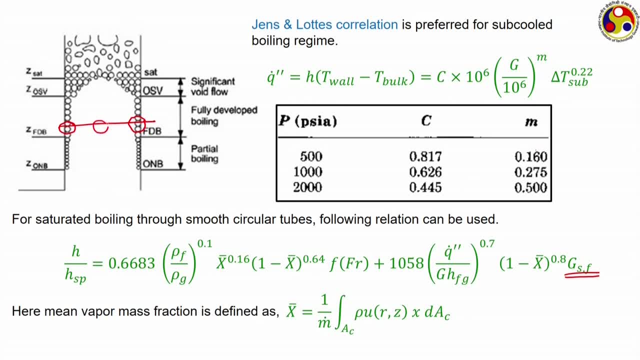 Or mass fraction. here also, you will be getting something, but if you take a sample from somewhere, you are going to get a mass fraction of 0. So you need to define an average mass fraction and this x bar value can be put here. This relation is applicable for x bar, a wide range. 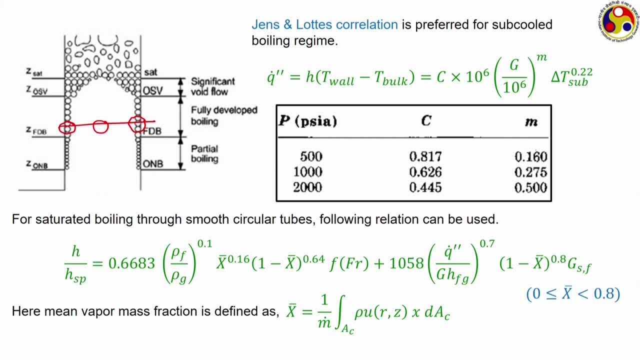 of x bar from 0 to 0.8.. So the choice of heat transfer coefficient is a complicated topic in not only in nuclear thermal heliolics but any heat transfer applications, as we had depending on experimental heat transfer correlations. So before picking one, we should be very, very 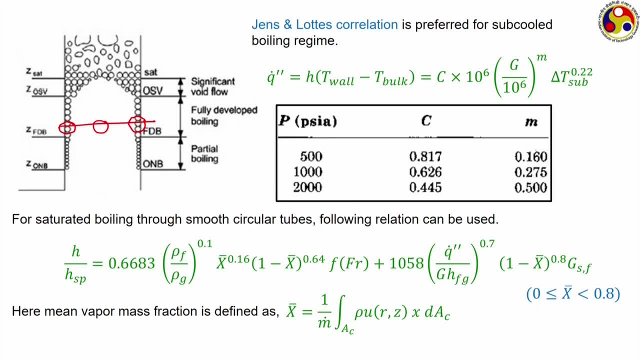 careful whether that is at all applicable for our case or not. Like in this, the last one that I have mentioned, it is applicable over a wide range of x bar, that is, 0 to 0.8, but say the situation you are dealing with, that is having a very high vapor mass fraction. 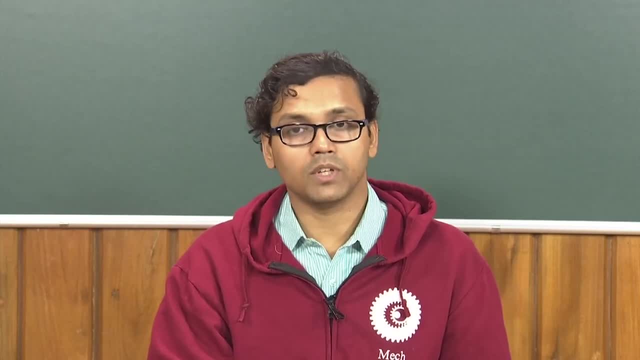 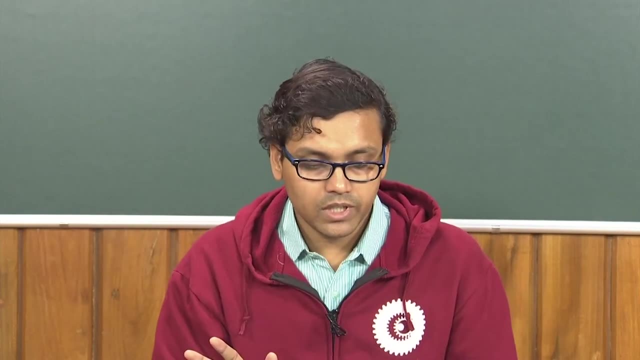 somewhere close to the channel outlet of your channel, which is something like 0.9.. Then this is not at all applicable. we have to found something suitable. So this takes us to the end of this particular module. Here we have learned about homogeneous. 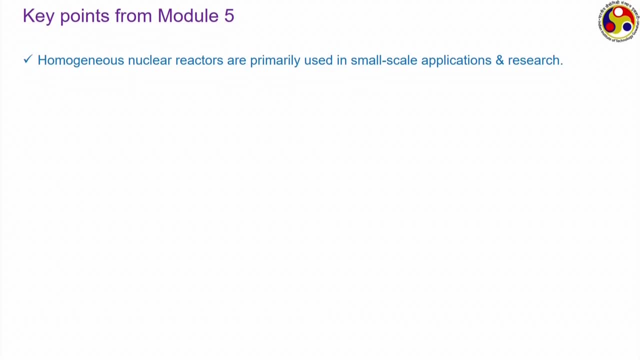 and heterogeneous reactors. We have seen that homogeneous nuclear reactors are primarily used forsmall scale applications, medical isotope production or hydrogen production kind of research. But heterogeneous reactors are primarily used inpower generation, where we have fuel and moderator placed in a repeated pattern of discrete bodies. 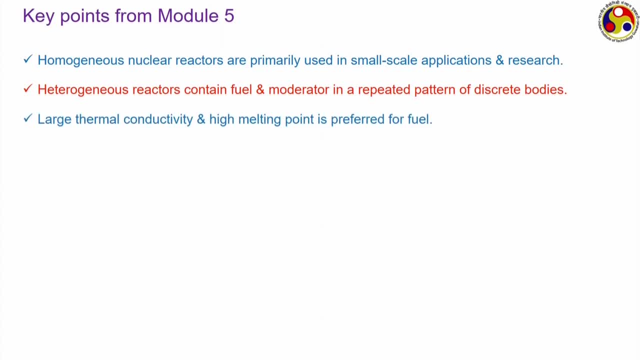 Now we have discussed about the desirable properties of fuel and cladding material. large thermal conductivity and high melting point is preferred for a fuel. Cladding provides a structural support to the fuel, and all can also aid heat transfer, particularly in gas cooled reactors. Then we have discussed about the energy that can get transferred, or that.